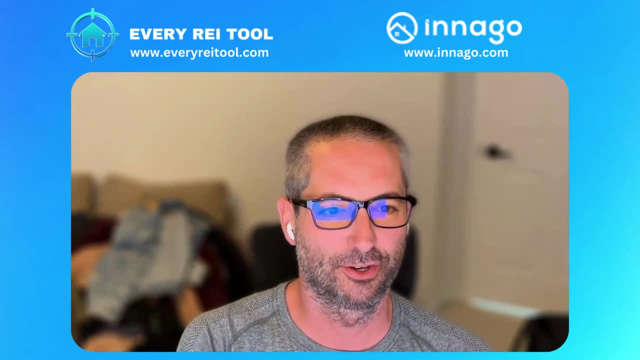 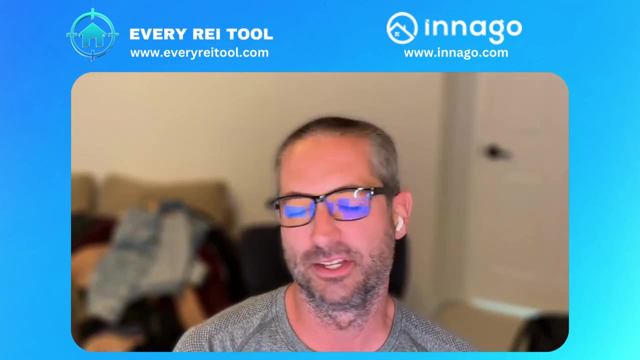 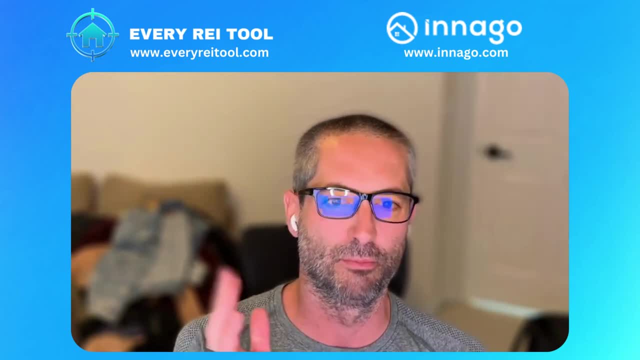 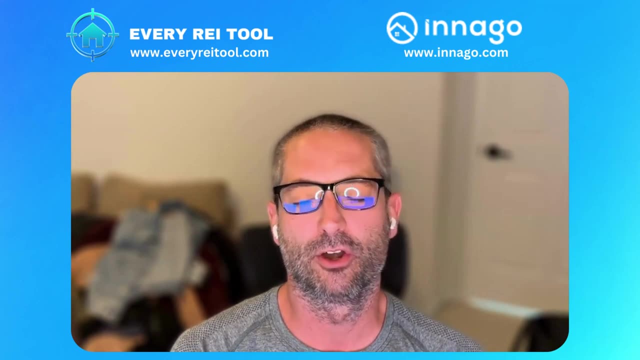 a good answer. I think it's a good answer. I think it's a good answer. And most tools available to real estate professionals and investors. there are multiple flavors or versions of those same tools. Is there a better like persona or target customer? Like who is Inago for? I guess. And then 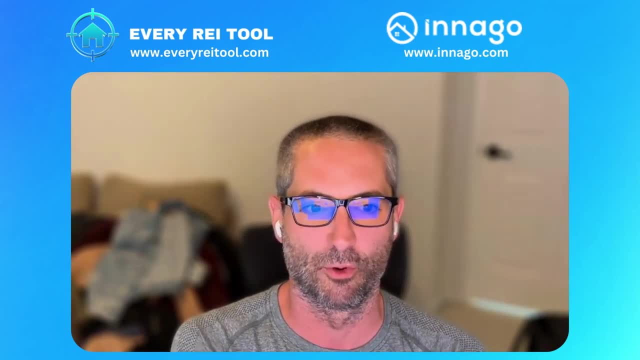 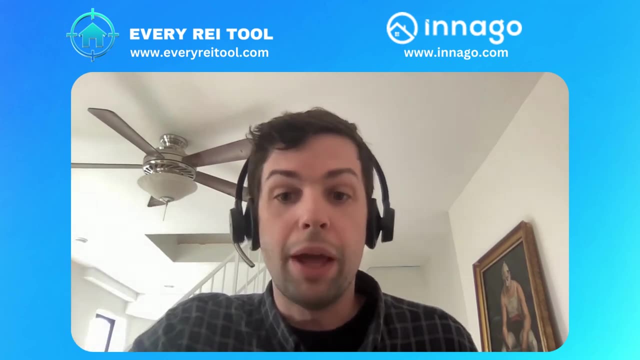 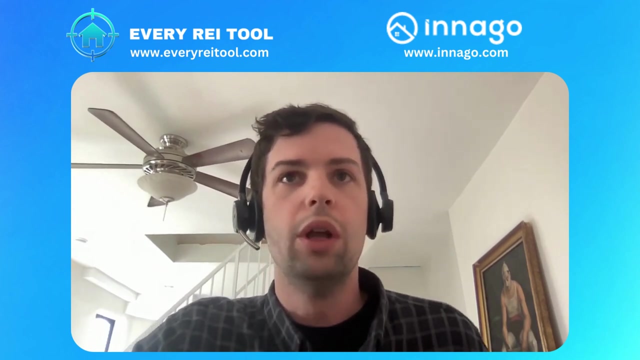 the flip question there is going to be: who is Inago not for? Yeah, great question. So Inago is really designed for those small to midsize independent landlords or smaller property managers that are working in a relatively independent manner. So we usually say anywhere from one to 100. 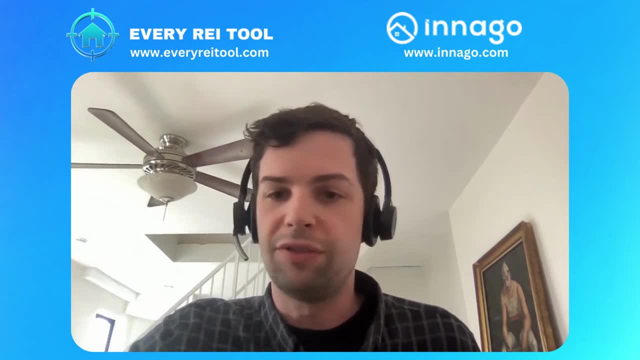 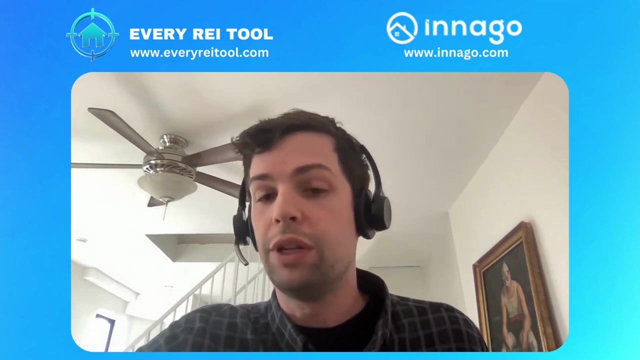 units. You know, if you're not typically managing a fleet of employees, if you, if you're in residential, commercial, those types of spaces, more traditional rental property, housing, is where Inago is going to be perfect. Inago is really not for the larger landlords, with one caveat to that. 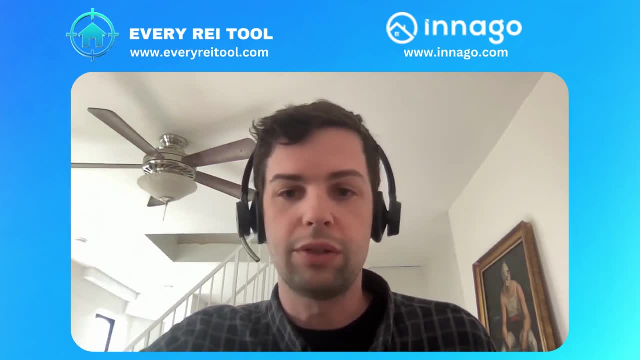 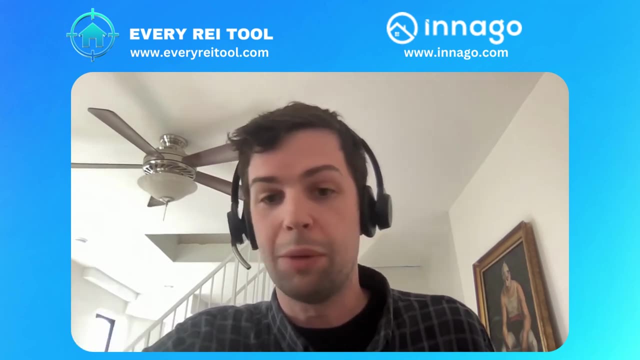 We do not usually work with landlords that have thousands of units. We do have a few exceptions. We offer integrations to some of the larger software platforms, So if you just want to kind of upgrade your tenant experience, you can use Inago as the. 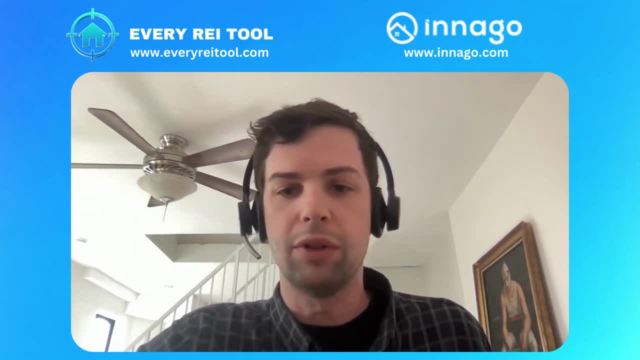 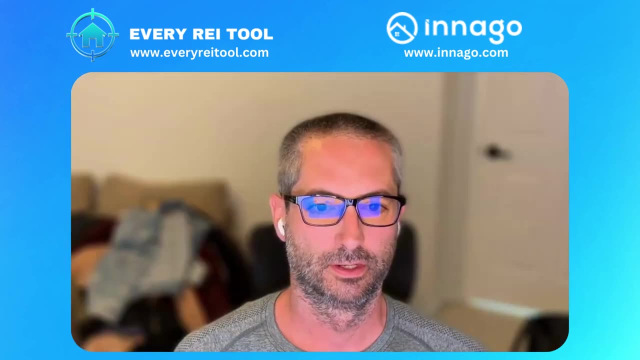 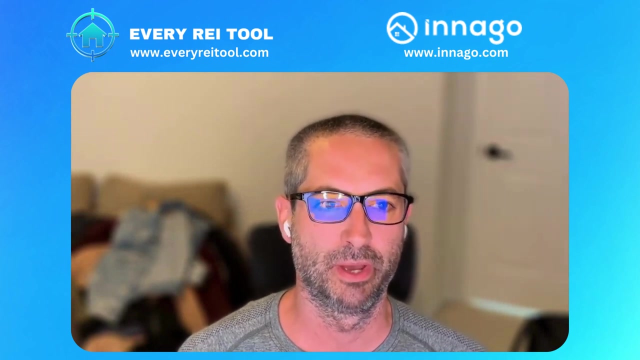 tenant facing side, But we are not going to offer the same level of features that an Entrata has or a Yardi has for those larger landlords Got. it Makes total sense, And you touched on this a little bit here. But one question that I always like to ask is: what do you feel Inago does better? 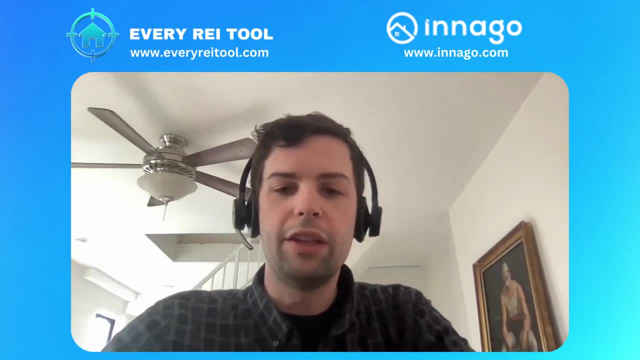 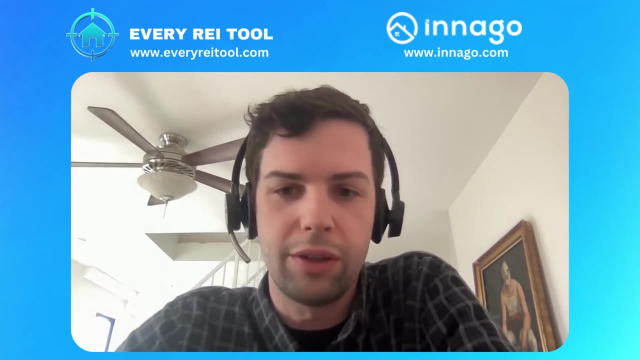 than other solutions out there. Yeah, I think it is that DIY piece, just recognizing that most landlords are DIY. I know it sounds like a really obvious thing, but I think there's so much software out there that kind of misses the boat on that. Can you say a bit more? Sorry to interrupt here, but can you say a bit? 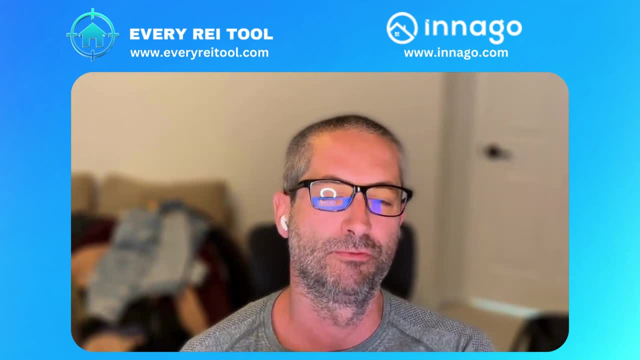 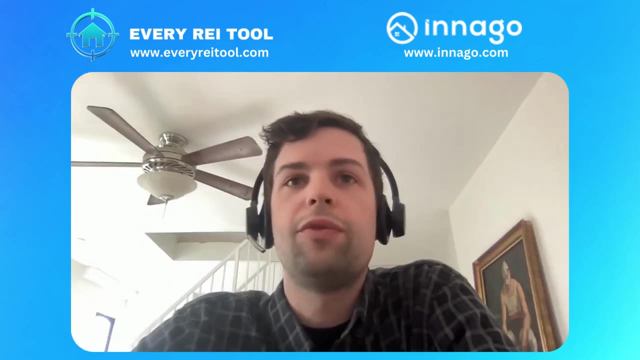 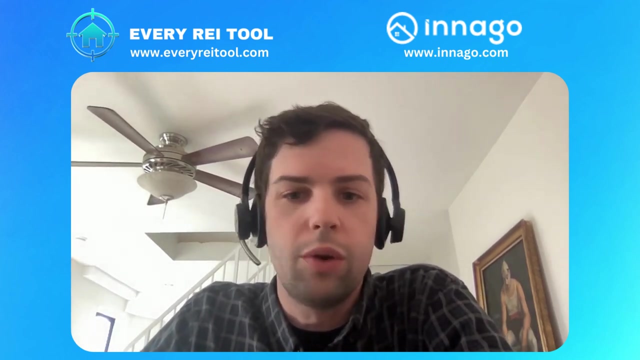 more what. what you mean when you say kind of you know features and aspects that Inago does better for that DIY landlord. Well, I think, fundamentally, landlords often learn as they go. Right It's, you didn't go to school to be a landlord. for the most part, That's what most real estate investors. 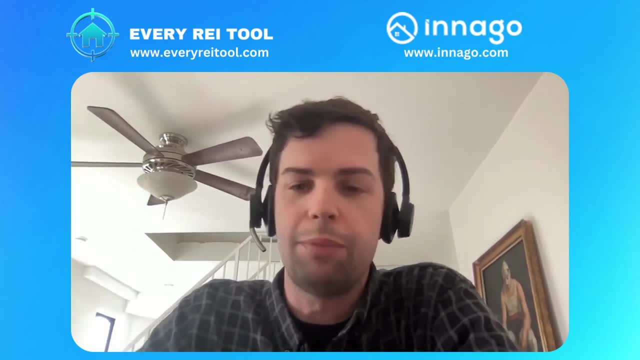 are: Yeah, exactly Like you have a successful nine to five job, You're an engineer, you're in sales or whatever it may be, And you say, hey, I want to set up my nest egg for the future, I'm going to start. 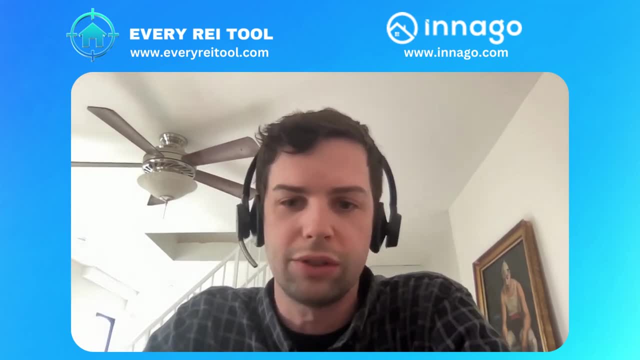 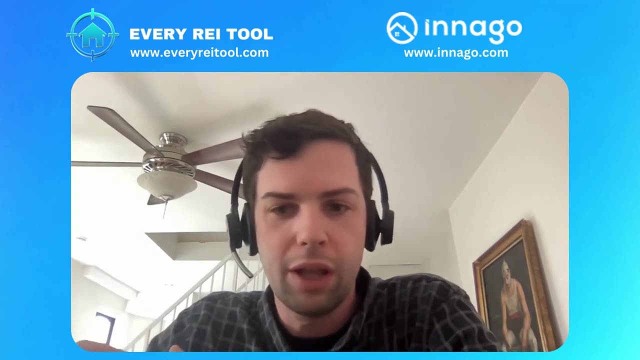 investing And you jump on bigger pockets or you start reading the books or the blogs or listening to podcasts or going to every REI tool to go do some research Right, And you cobble together your own kind of formula of building your real estate portfolio and managing that portfolio And yours. 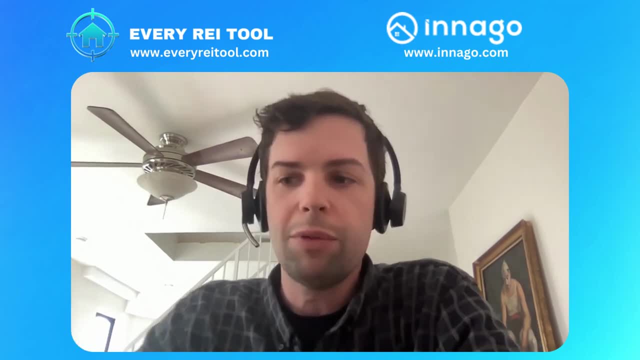 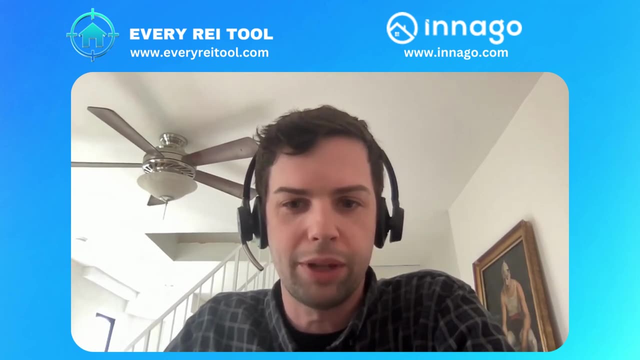 is going to be more structured and approach and flavor than the next person. So everybody is really unique in the real estate space. It's not as much. it's not like you know, gap based accounting, where the rules are really tight and set in place Right. Your late fees may be different, The way that you 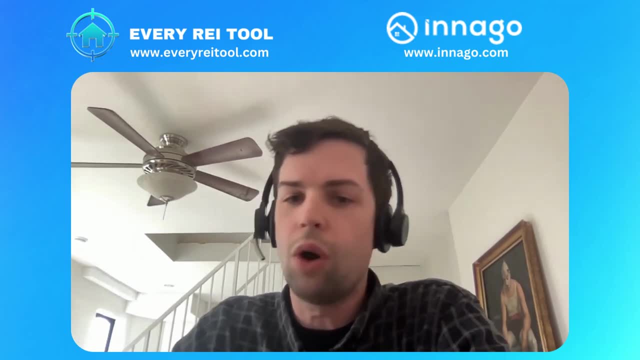 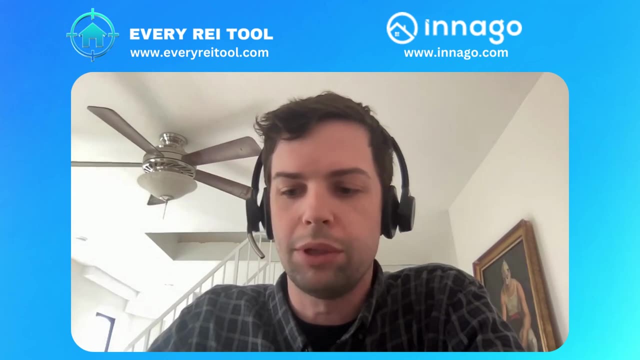 collect rent, whether or not you allow partial payments, you know your different documents that you use, all these these teeny tiny variety of little decisions and requirements that you have is going to be completely different the next. So what we tried to do is balance the fact that A this: 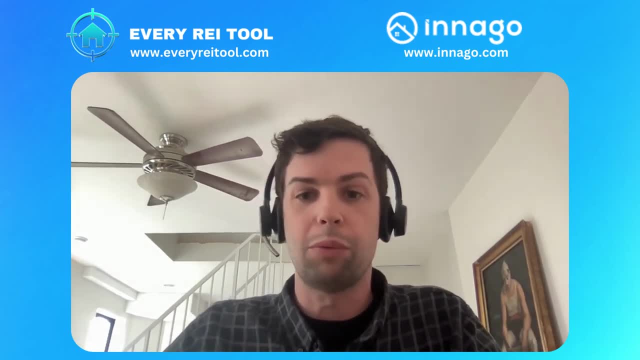 landlord persona doesn't have a lot of time to learn a super complex software But by the same token, that software has to be flexible enough to deal with these different structures and setups. So we have spent, you know. I'd say it's taken us long, It takes us longer to release a feature. 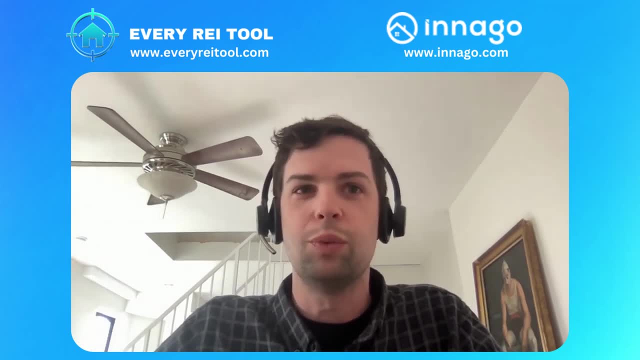 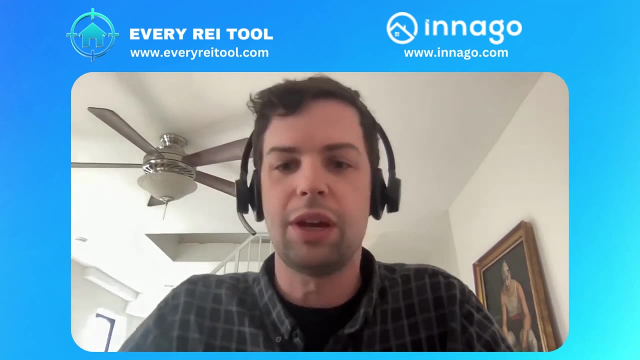 than most any other software in our space, because we try to think of it from all those different angles and make sure that it's including the different types of landlords and different types of DIY landlords. So that's a subtle thing that's hard to articulate and point at a specific feature. 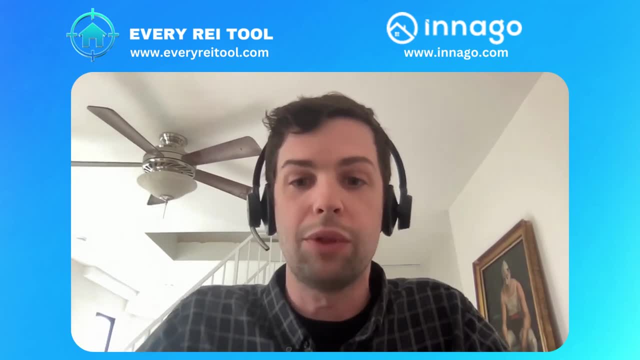 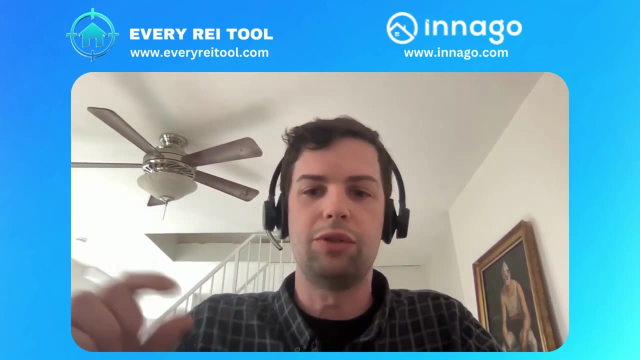 and say this is the killer one that we have, that others don't. But I think if you play around with Inago for a little while, you pick up on it really quickly where, oh man, they did kind of think of a subtle but intuitive way to address my proration or to address rent escalations or to address my. 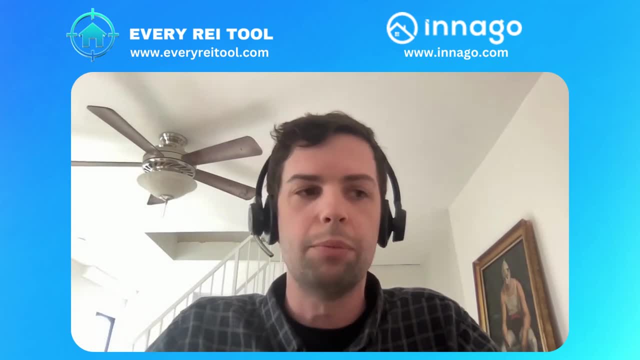 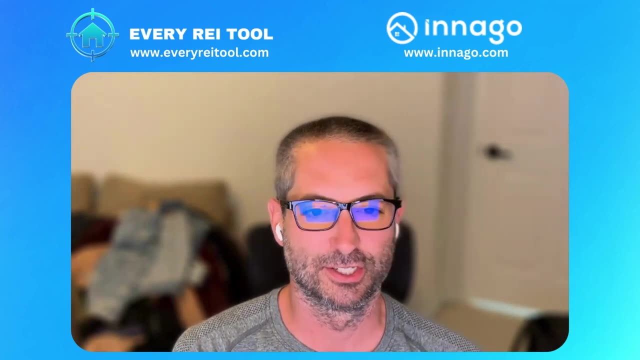 various you know crazy late fee structure that I've set up here. So I think that's really the big difference. Yeah, Awesome, And like we were talking about before we hit record here, I'm in, you know technology and software by day and I can appreciate how hard it is to keep or to. 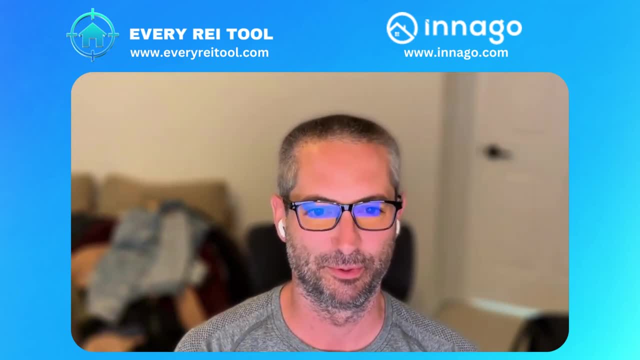 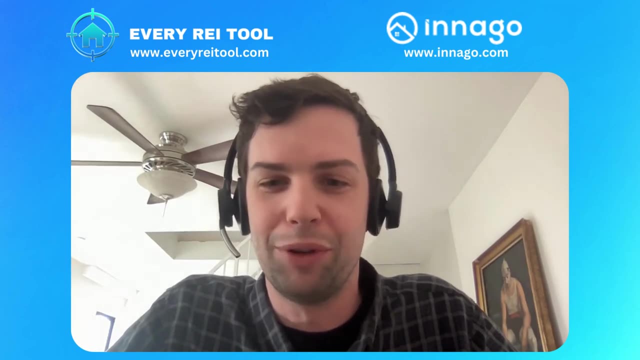 build something complex yet keep it, you know, intuitive and simple to use. Yes, we certainly have made the wrong call a lot of times, but we're always learning from the wrong call and improving on the next one. you know, but it is tough, And you touched on this earlier as well, but I'm not. 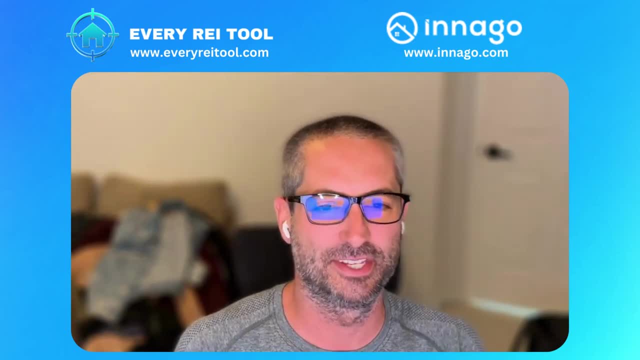 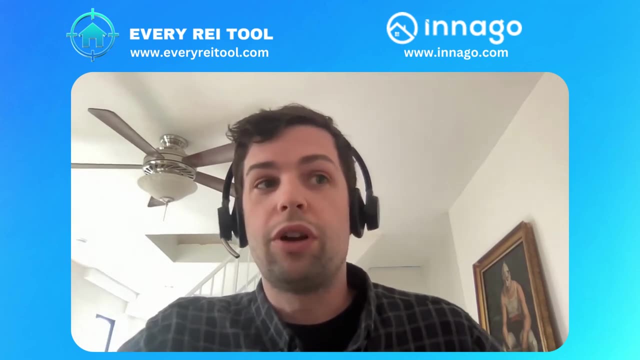 sure you know people. I guess people need to hear this again. Did you say Inago is 100%, completely free? Is that the price point? Yeah, that's the price point. We don't charge landlords anything. We charge for a few kind of. Value driven features within the software. So, for example, when a tenant pays rent online, the tenant is going to pay $2 if it's an ACH transaction and they're going to pay 2.99% if it's a credit or debit card transaction. Most other software out there, even the ones that 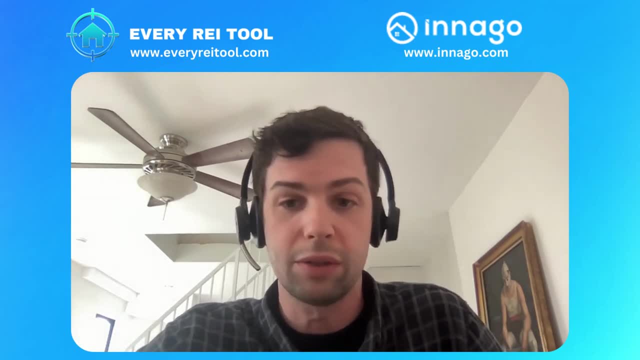 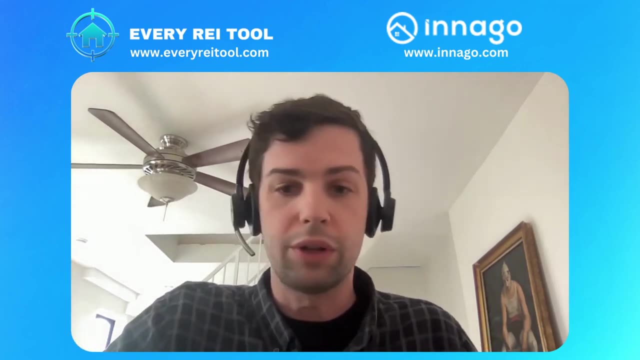 charge you a monthly fee, are still charging those fees for the transaction, sometimes higher than those fees. So it's just tied to those online payments. We also charge if you screen a tenant through Inago. we're going to charge the applicant If the tenant buys renter's insurance through. Inago, we get a cut. So we found different ways to kind of monetize the experience without hopefully putting too onerous of fees on any party that's involved. I love it. Well, free for landlords, I'll take it. I love it. Yeah, Awesome, Sounds wonderful. 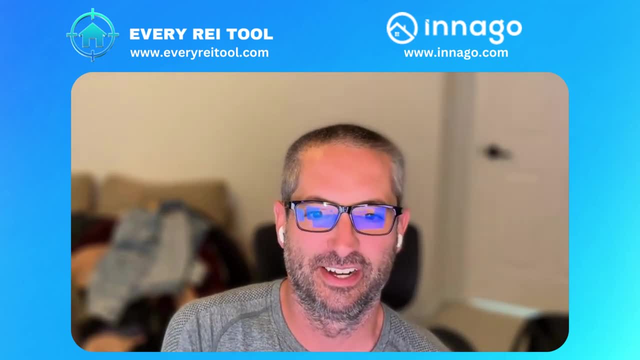 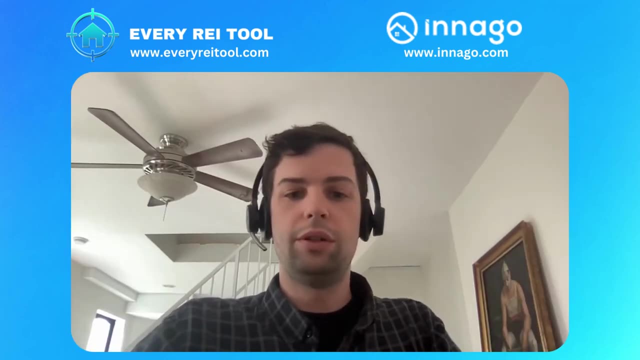 For why don't you, if you could, you know, start sharing your screen here? And why don't we just jump into the demo and see what this awesome tool is all about? Yeah, let's do it. Just get it zoomed in here, Cool, All right. So this is the Inago dashboard. I have my 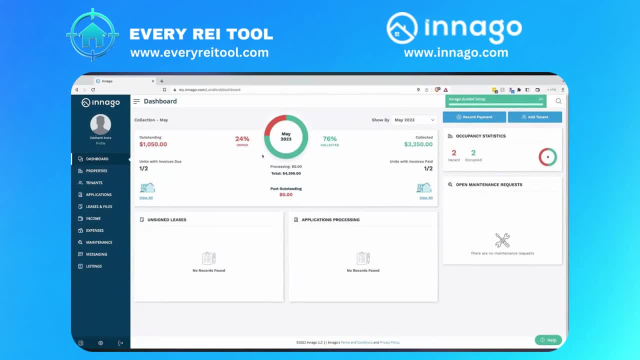 location landlord set up here. This is Siddharth Aurora of Aurora Properties. Siddharth has one building actually, with four units in it. You can see it here: Main Street Lofts. This is Siddharth's dashboard And from here he can see how his collection is going. 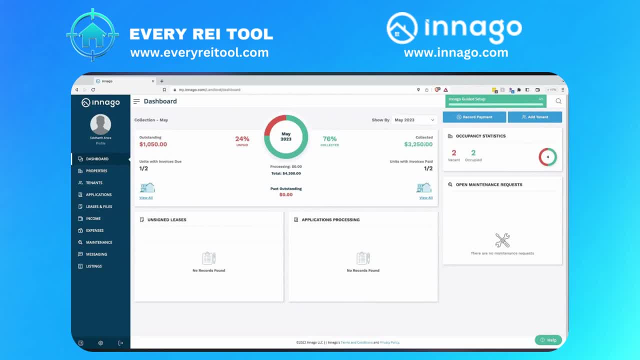 this month. right, It's showing us May by default. We can see what's collected, what's still outstanding. We can click on this and jump right into it if we want to see who owes money. If we had some documents that are in the signing process, those will appear here under unsigned documents. 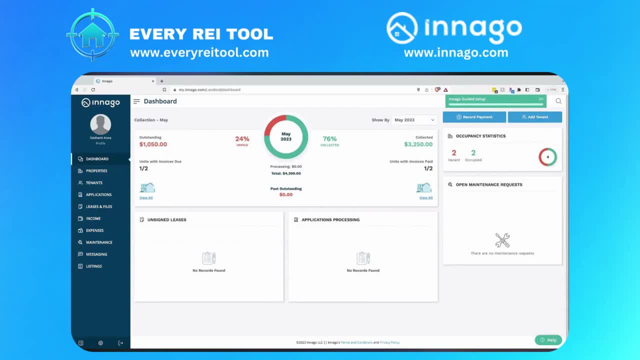 Applications processing, if you're screening anybody or collecting a basic application, If any tenants had put in maintenance tickets, what your occupancy statistics are, et cetera. We really wanted to make it so that all the important information is up front in a really streamlined 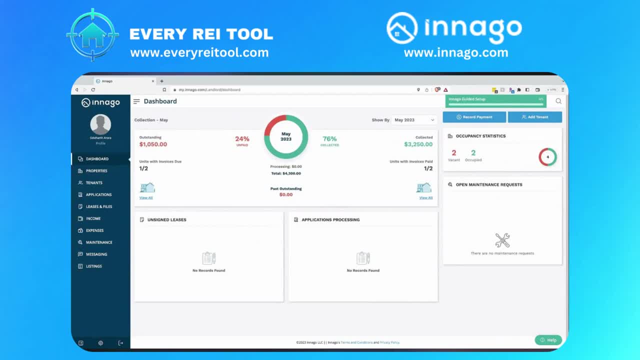 kind of simple, not overwhelming, way. I've seen plenty of dashboards where there's like a million statistics and you don't know what to care about. We try to keep it really focused here, but also give you a relatively comprehensive view and an easy launch point to various other features. You 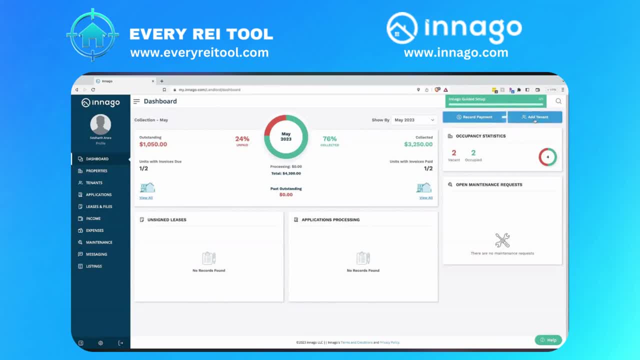 can quickly record a payment that you received offline. You can add a new tenant to an existing lease or a new lease within Inago. It's easy to access a lot of different features and requirements that you might have at any given time from this one place. 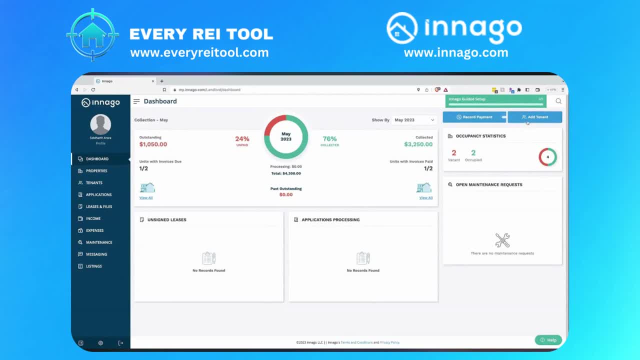 Speaking of adding a tenant, I think it's really useful to go through this particular feature because it's so core to any rental property management software that you use the actual process of getting the tenants set up- Hopefully once they're set up, and added most of the rest. 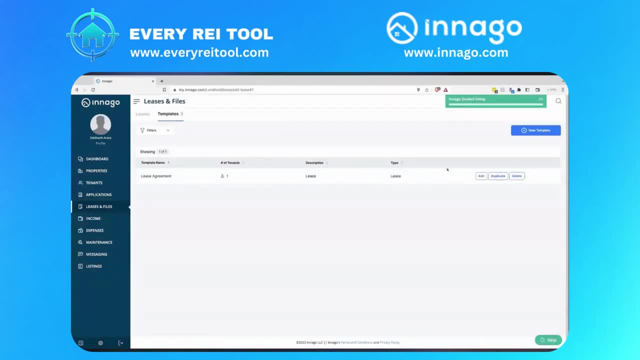 of it's pretty, set it and forget it. So this is kind of the important bit here I'm going to go. let's see here. Hang on one sec, Nathan. quick aside: here I am using- we're launching a new Here. I've got a list of all of my units. I can see some that are available. 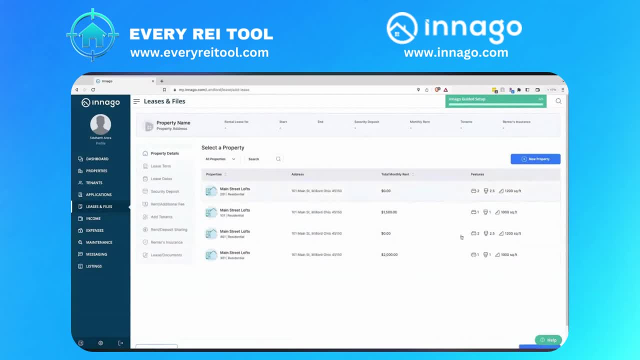 some that are not. I'm going to go ahead and select unit 201 and we're going to add a tenant to this particular property. First I can choose what kind of lease term it is fixed, or month to month, Let's say month to month for this piece of property here and then on the right side of that. 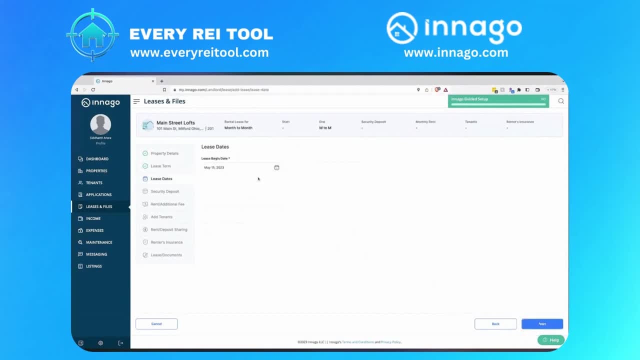 I can speaker, Then I can source some of the property to be onto a previous성을 service. So this one, we'll say our lease begin date is today. they're ready to move in right away. we set our security deposit. we can set our security deposit due date. let's make it today. 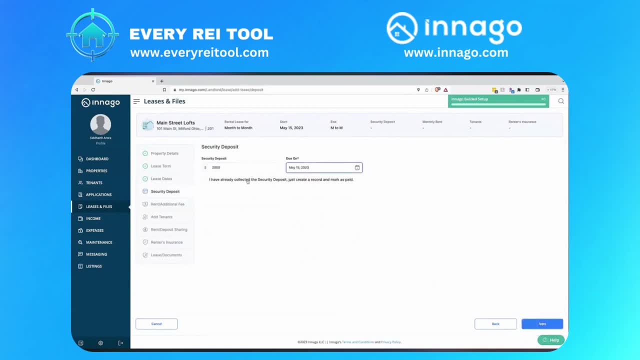 and actually, hey, they handed us a money order already, so i'm going to mark this as fully paid. now you can see we're we're trying to keep this really streamlined. there's not a ton of options on the screen for you. it's really focused. it's it's difficult to to get lost on, you know going. 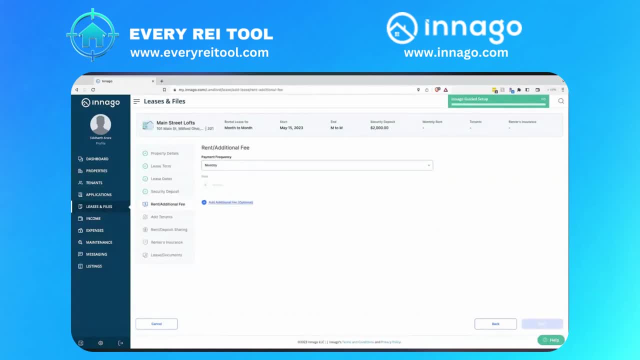 through this sequence. so let's say it's a monthly lease. yeah, go ahead of the step-by-step guide. on the left they're kind of walking through. each step makes it super intuitive, exactly, and you're getting the summary of the lease that you're building at the top. so if you made a mistake, 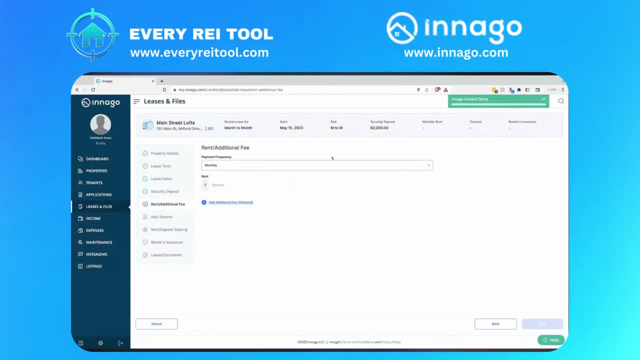 or you're forgetting some piece. you can see it right there the whole time. so we can set our rents amount. let's say it's 2 000 bucks. we're going to make it due on the first and we'll say that the first invoice is due on may 15th. now i mentioned one of the things that inago you know. 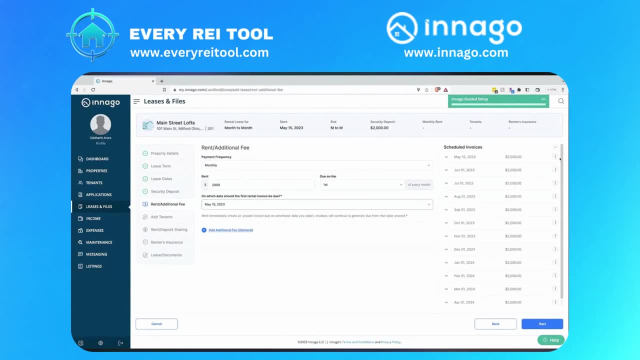 one of the kind of those diy quirks or those little things that inago makes simpler is proration. and here on the right side of the screen we have our rent schedule that just popped up. it's showing us the next 12 months of rent. i can go to may 15th. hey, they're moving. 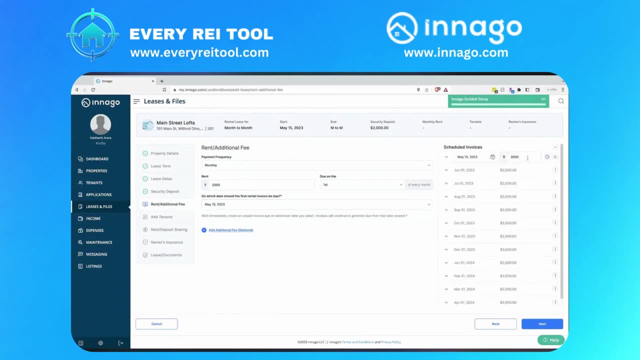 in halfway through the month. they're not going to pay the full rent, they're actually just going to pay half. so we're going to drop that down to a thousand and prorate it right there now. we don't want to assume that you prorate half because actually, technically they're living there more. 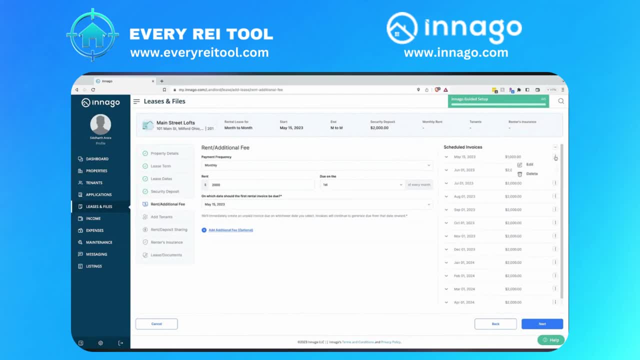 than half. so maybe you're somebody that prorates by the day, so i could adjust that to a different rate. i could totally delete this invoice. i can change the due date. i can move my last month's rent due my first month's rent. i can make all sorts of little tweaks and changes here to that rent. 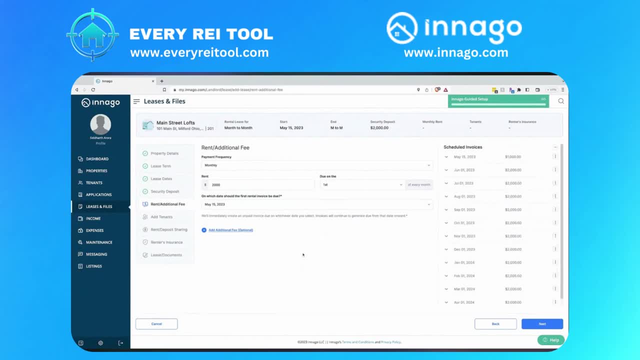 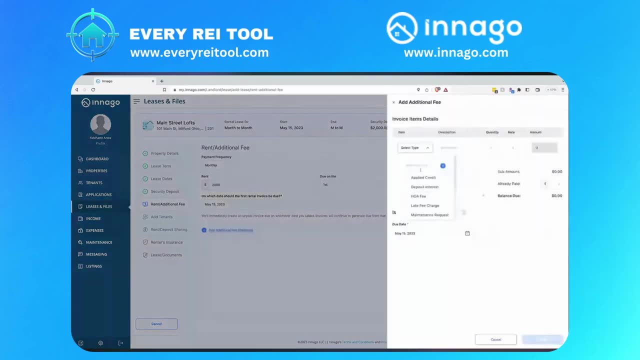 schedule while i'm going through this process. likewise, i can create additional fees. so if i need to charge like a pet fee for them, for example, a monthly pet fee, i can create that recurring invoice right here as i'm going through the setup process. so super easy to add additional fees. 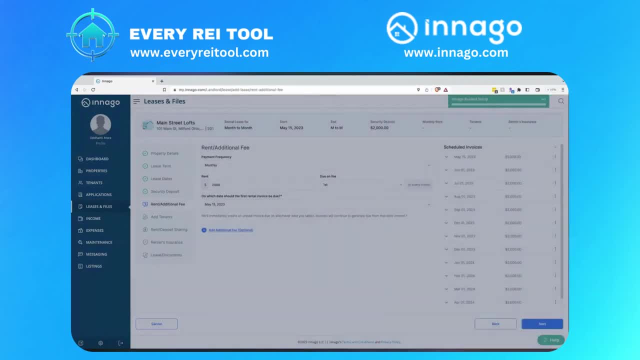 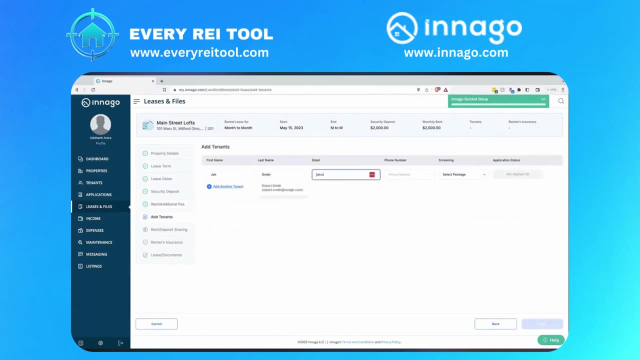 whether they're recurring or one-time charges. yeah, awesome, next up, i'm going to add some tenants. here we go. oh, we already had a john smith in the system, so we'll go with him and we'll say that the screening is not required at this time. so i've already screened him. i've already taken a look at. 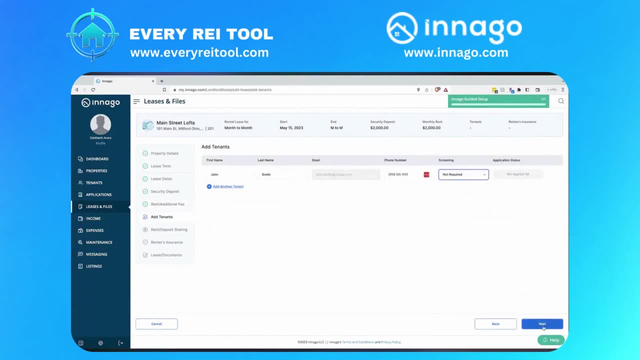 him. i'm not going to move forward with that. um, i can set my rental split. if i had multiple tenants. this becomes a little more relevant with one tenant. he's going to obviously pay the full amount. i can say, hey, i'm not going to let him make partial payments, i want him to pay the full amount. 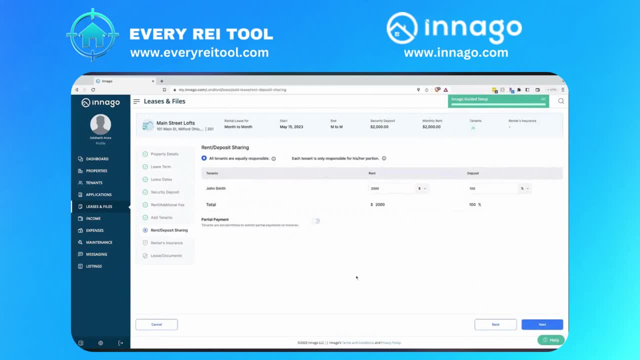 every time. yeah, so that's what we're going to do. let's go ahead and set up a rental split to the rental split. i want to set up a rental split here so i can see how much i'm going to pay. move forward, decide whether or not you want to request or require renter's insurance. 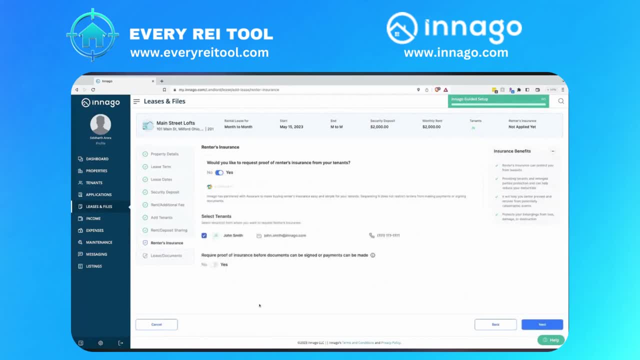 So I could say yes. Now it's going to send him a request for renter's insurance that he can either upload a copy that he purchases elsewhere- He doesn't have to buy it through Inago- or we make it really easy for him to grab a quote, see what the price is and, if he agrees to it, purchase that. 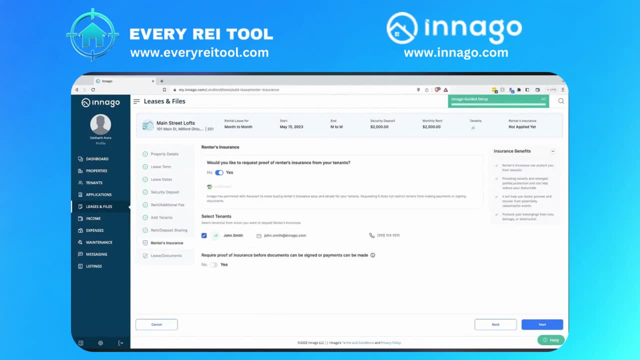 policy right then and there. So it's really easy to manage renter's insurance, which is a really important tool that landlords use to kind of mitigate risk on their end. And I'll say that it's required before he can sign a document. Next up is the document signing phase. Now, Inago. 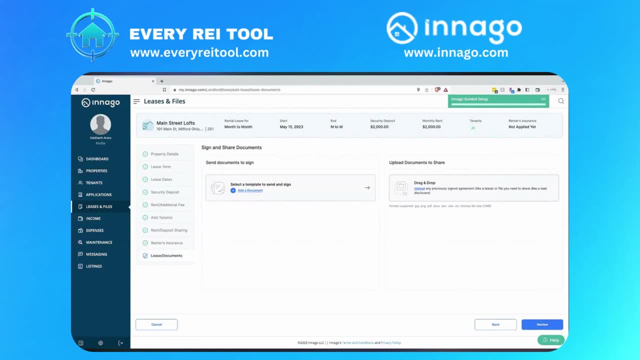 works with HelloSign- or, I guess, formerly HelloSign, now Dropbox Sign- for the actual signature process, But we built a whole bunch of tools on top of their existing template creator to make it even easier, specifically for landlords. So, whereas in Dropbox Sign you basically have five fields to 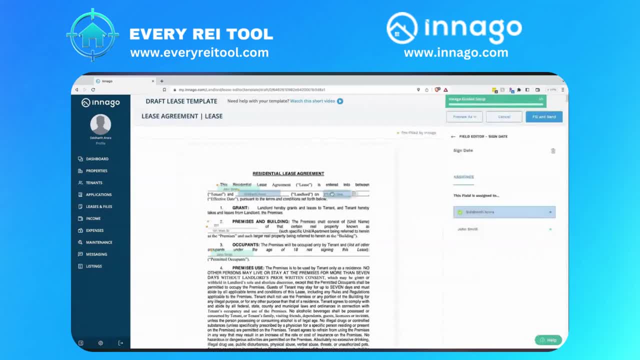 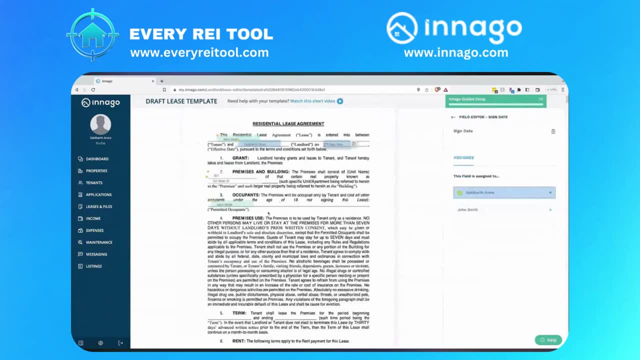 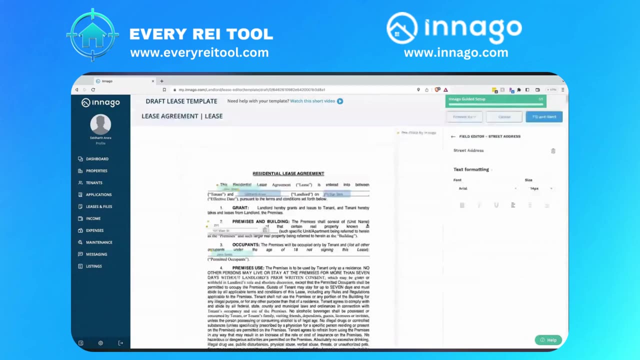 choose from. We added a bunch of additional ones. We have the sign date, of course, but we also have fields like the rental amount or the unit number or the street address right. These are fields that don't make a lot of sense within HelloSign but make a ton of sense within rental management software. So you 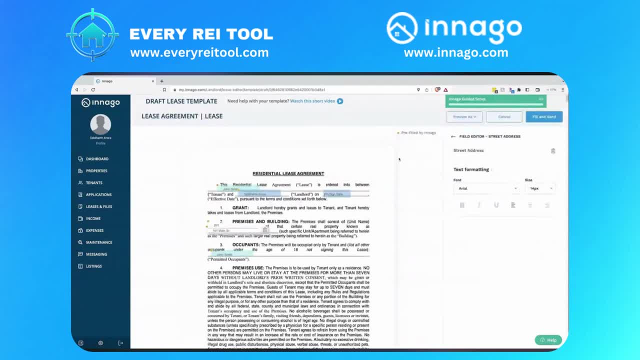 can choose. you can drop in all those fields that you need. drop in the signatures, upload a copy of your document again, whether it's a lease or some other agreement, and you can send it off to be signed. So I'm going to hit fill and send. 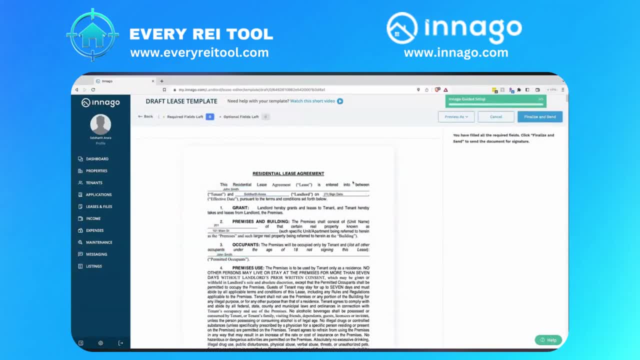 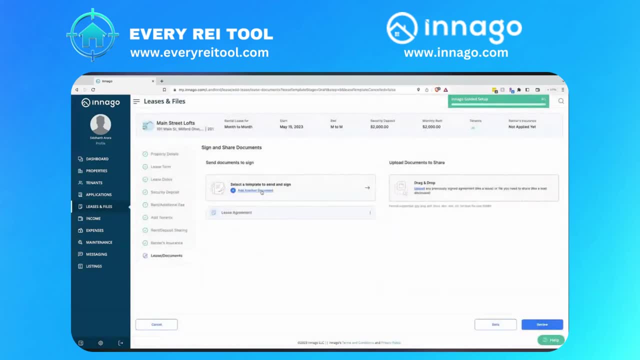 Looks like there's no fields that I have to fill in before sending, so it's allowing me to proceed, And now I've uploaded that document to be signed. I can also add another one, though, right, Maybe I'm not just signing a. 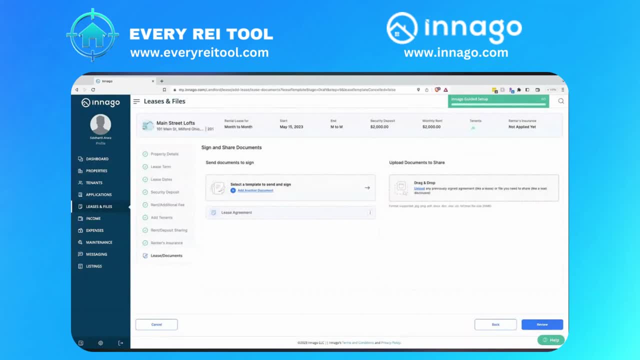 lease, I'm also signing some addendums. Well, I can click sign another document And I can fire those off. Looks like I got an error that said I can't, but I can. Okay, then I can upload additional documents if I need. 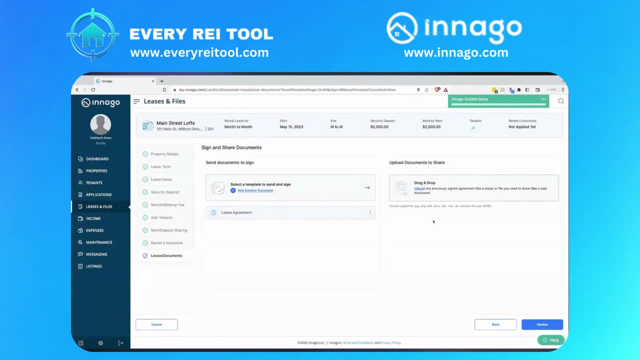 to whether it's like a lead based paint Agreement or something else that you need to share with the tenant. you can upload those as well. So all of your documents signing, all of your document uploading you can, you can add here and you can send those off. So final step, 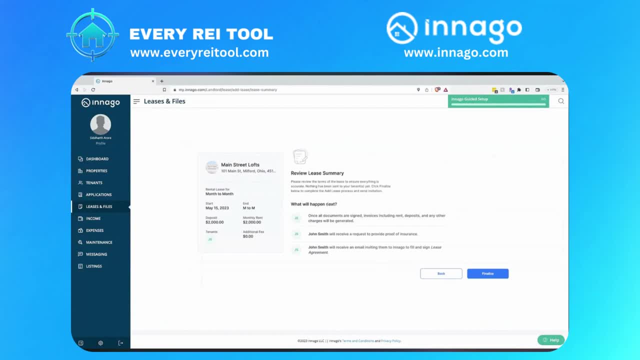 here I'm going to review everything I've put together. it's going to tell me clearly what's going to happen next: sending these off to be signed. once they're signed, you know, all the invoices will be generated, etc. So I can hit. 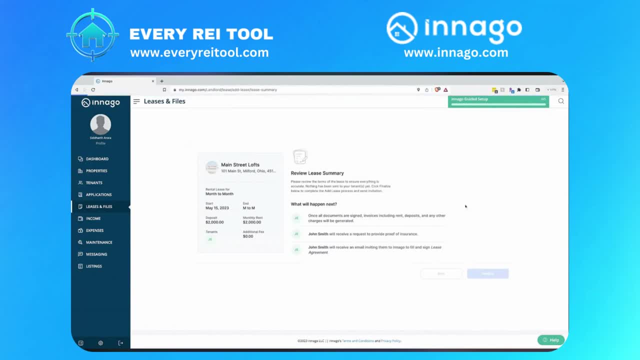 finalize And I've just added John Smith to my Inago account. So now I've got John Smith listed here in this month to month lease In process, because he hasn't signed it, of course, but he's added in here to Inago right alongside my active leases. 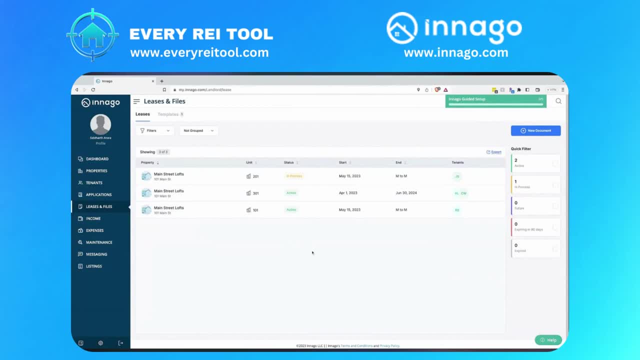 And then I'm assuming they obviously get notified of this, you know, by email, because you had John Smith's email, and then they can go in and take pick up the process from there to to get this thing closed. That's exactly right. Yep, they're going to get an email. they'll get reminders. they can sign it right from their phone or 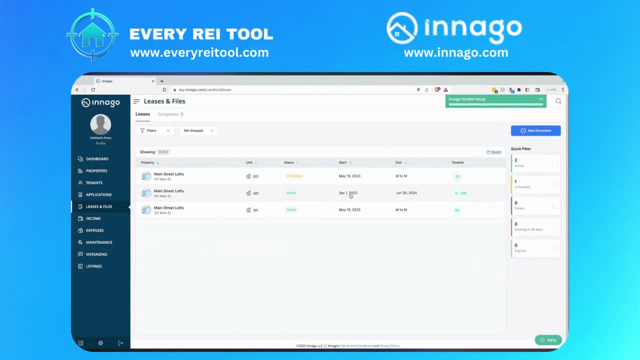 their computer whatever's most convenient for them, And then we'll notify you, of course, when they've signed. Now I could go in and sign this document right now, if I want to. Some landlords choose to wait until after all of the tenants have signed with a digital document. it's not valid until everyone. 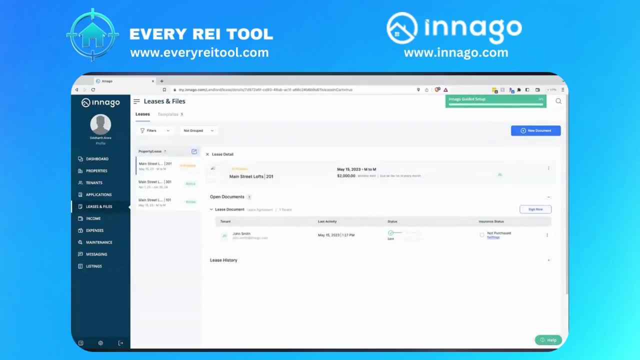 signs anyway, but it's totally up to you: sign it now or wait until you get that notification and sign it once they're done signing. however you want to handle it. Yeah, I think you mentioned this and I see this on the on the site as well. We're obviously in the web experience here, But I 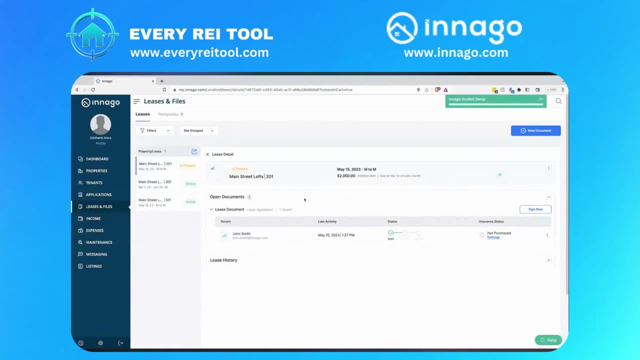 believe you have a mobile app as well, or a mobile experience at the very least mainly, for I would assume that's what tenants use the most is like the mobile experience. Yeah, we have both, Both the tenant mobile app and a landlord mobile app. So you can- you can log in as landlord as well. take it with you on the go. We also 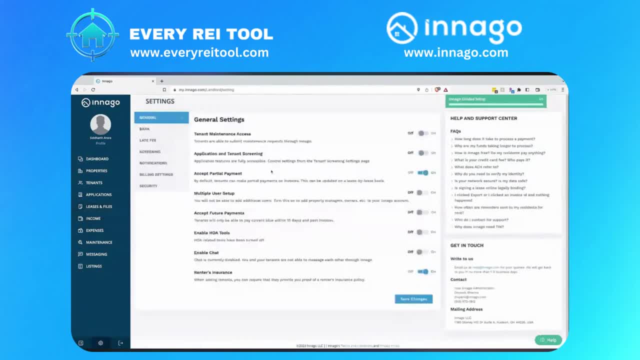 support sub users in Onago. So if you do have additional employees or team members that you work with, it is possible to give them access. So I'm turning this feature on for this particular landlord. Now I have this users page And I could add somebody like a maintenance. 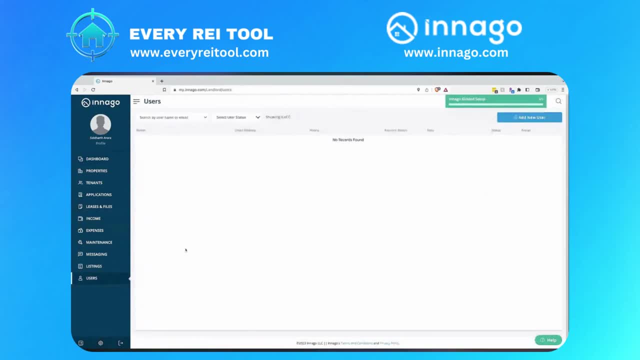 person, or a property manager or a leasing agent, and give them access to specific features. They can also log in using the mobile app, which is, you know, great, depending on kind of what their role is. All right, so that's, that's how you go about adding a tenant, which again is kind of the bedrock of any rental management software. So 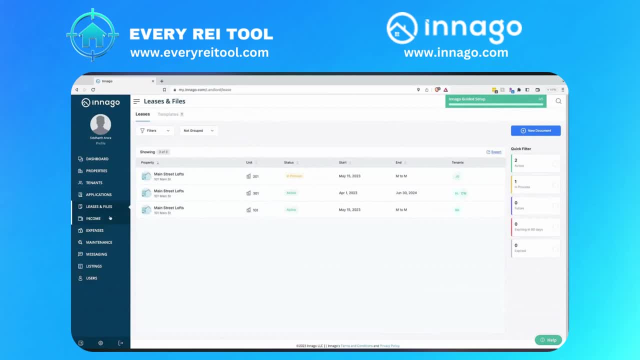 hopefully you know, you can see how simple and straightforward it is but also how balanced it is. with that, that complexity and different potential, you know questions or requirements that you have as a landlord. So let's take a look really quickly at the income page, Because 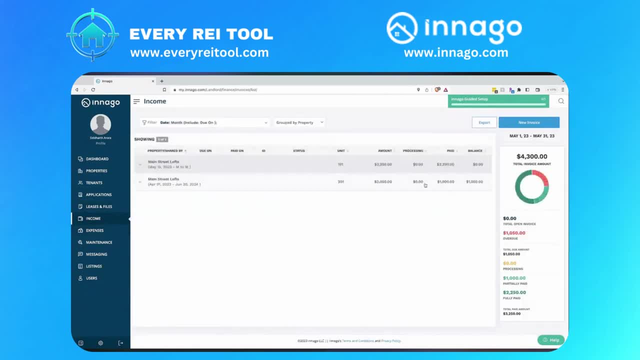 of course, that's what you really care about when. when you're renting out properties is is is the cash flow that it's generating for you. The income page is always filled with a lot of information. The income page is always filled with information. 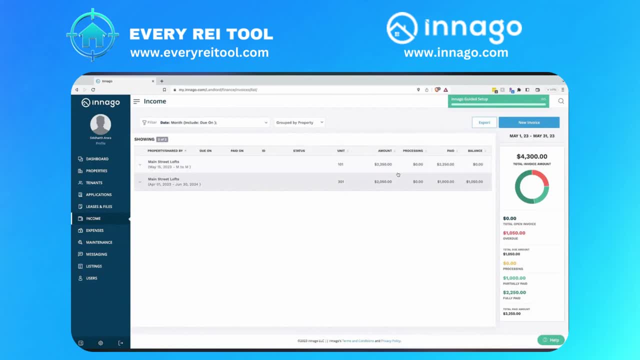 The income page is always filled with information. So when you are renting out a property like a home or home establishment, you're short on cash. You have to pay in cash, so you need to pay in cash every month. So every month it's a different type. 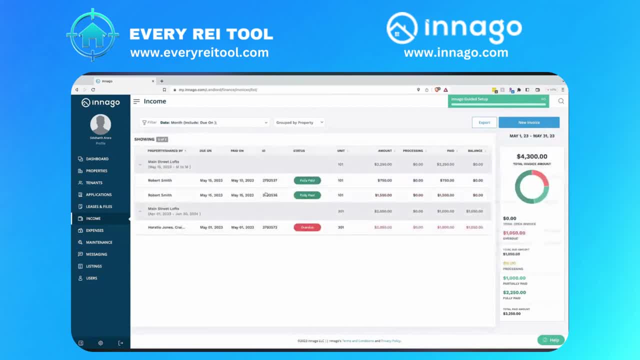 see, we've got a few different invoices. we've got robert smith, one of our existing tenants. looks like he paid his rent and his security deposit. looks like he was also paying some sort of pro rated rent there. and then we've got horatio and craig, who are living in our other unit, and they 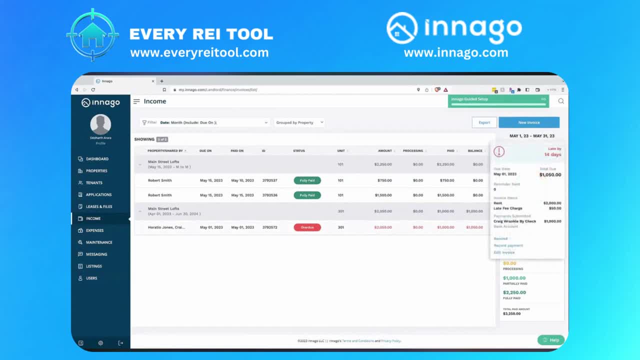 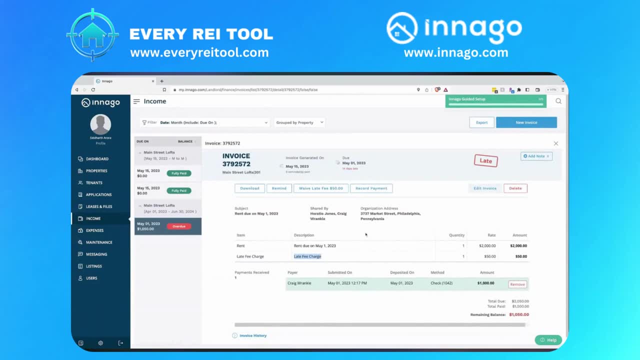 have not paid, or at least they haven't paid a portion of their rent. so we can look at this invoice and it appears that inago's already added a late fee charge to this invoice. that happens automatically, you know. if we're feeling generous, we can quickly and easily waive that late fee for. 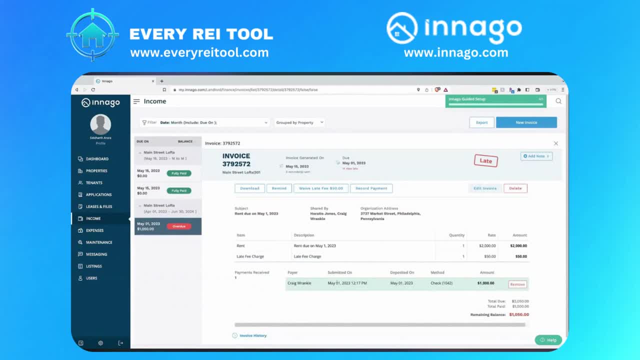 them. we can see craig made his payment. horatio has not assuming they're splitting it and we're allowing partial payments. um, now both craig and horatio are notified of this late invoice. it's not like just horatio gets notified because he hasn't paid his portion. both are aware and both. 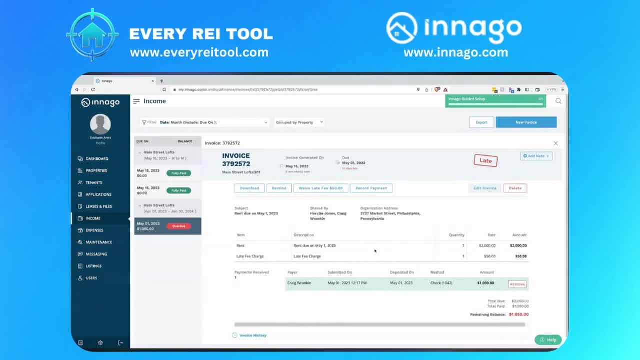 are held accountable for that. um, so it does keep them honest as, uh, as tenants under a group lease. um, some other things you can do here, of course. download a pdf version of this. you can send an additional reminder. we're already firing off reminders for you. you can waive those. 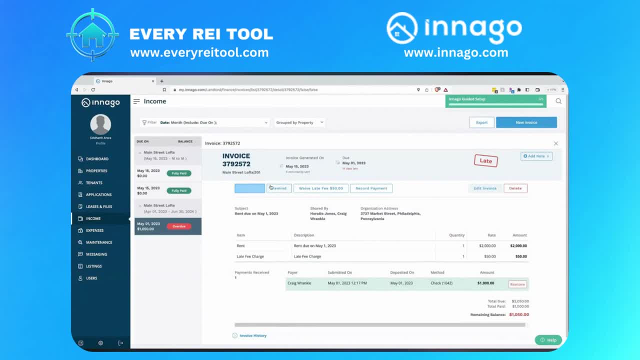 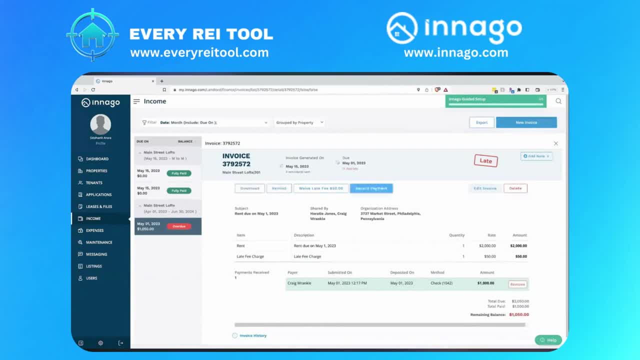 cash, etc. you can edit the invoice so you can add additional fees if you need to. you can also add credits. so if, for whatever reason, you say, you know, uh, somebody takes out the trash for you every month and you're going to give them a credit now, this will be a whopping credit for taking out the 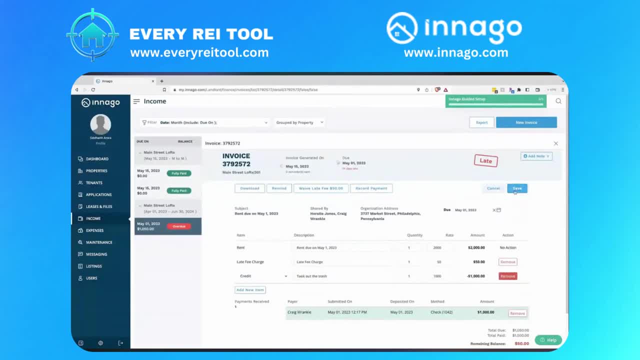 trash every month. but you know, you could give them a thousand dollar credit, exactly, you give them that thousand dollar credit and, uh, go ahead and waive that late fee and hey look, they're, uh, they're all set, things are looking good again. um so, yeah, lots of flexibility, lots, lots of control over these. 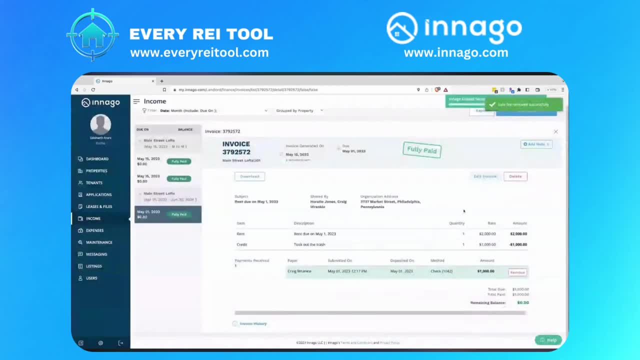 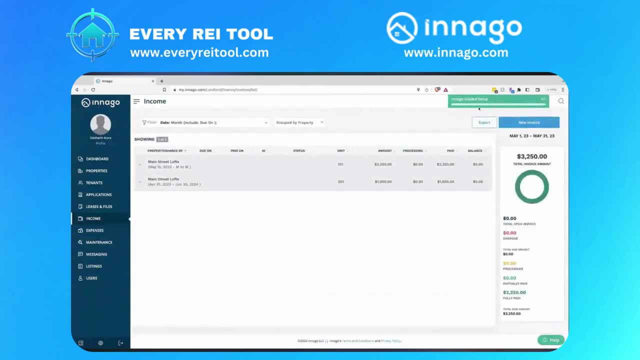 invoices, um, you know, even after they've been generated there. yeah, no, it's super clean, cool. um, one quick note here: um, basically every page in inago has an export button. on it. it's your data. you can get it whenever you need it. so you can click this export and it downloads a nice clean. 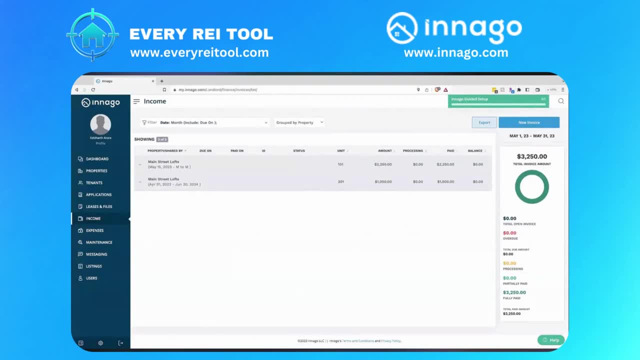 csv file for you that you can pull into other programs you know. store for yourself, manipulate, if you know you're doing some advanced pivot tabling or something. um, really easy to get access to, uh, to that data. yeah, i don't want to jump ahead here. if you're. 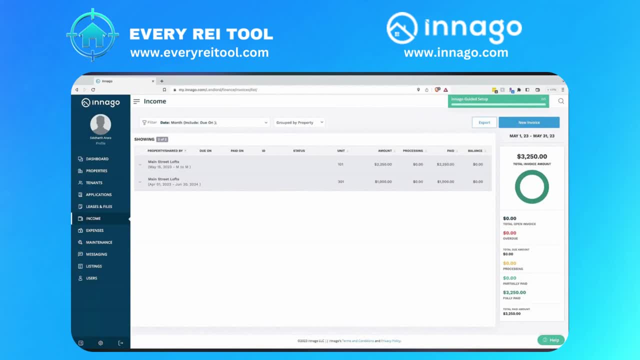 going to get there. but i'm curious because i see you know expenses here. we're talking about you know leases and exporting data and stuff like that. what's sort of like um reporting functionality does inago have? like, if you wanted to, you know, start sending stuff to your? you know cpa or you. 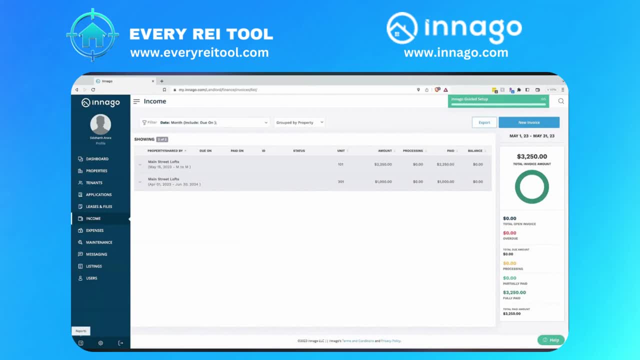 know, do your end of year taxes, stuff like that? yeah, that's a great question. so i i have a very small, very modest portfolio. i have eight, eight units that i own and manage myself and i use inago exclusively. i don't use quickbooks or any other sort of software, but i do want to note that inago 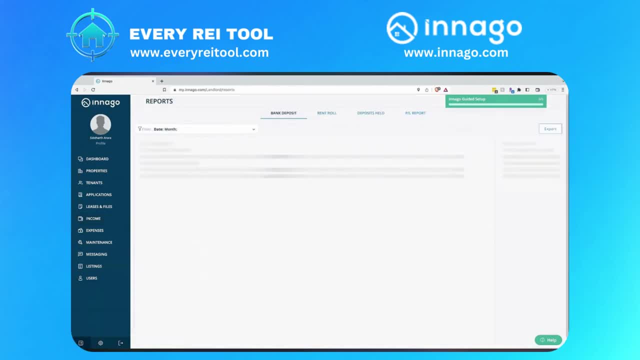 is not full accounting we we don't intend to be. we have a variety of different reports and for me and for my cpa they're perfect. it makes life so easy. at the end of the year, i download, i export all the data from the income page for the year, i export all the data from the expenses page and i go to. 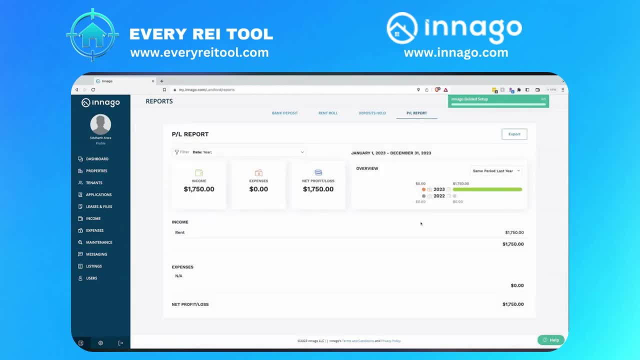 the reports page in inago and i export the p l report, the income report, and i fire those off to him and he's got everything he needs. now he often comes back with you know he's got everything he needs. now he often comes back with some questions like hey, you miscategorize these. you know right, exactly, uh, but there's not a lot of. 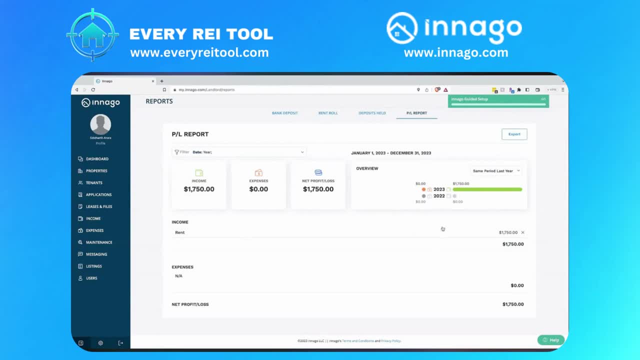 software that's gonna solve that problem for you. so yeah, we have a great p? l report here and it is interactive and dynamic. so, for example- and there's not a lot of data for this- you know test landlord here, but if i click on rent, it actually expands and shows me all of the different invoices and 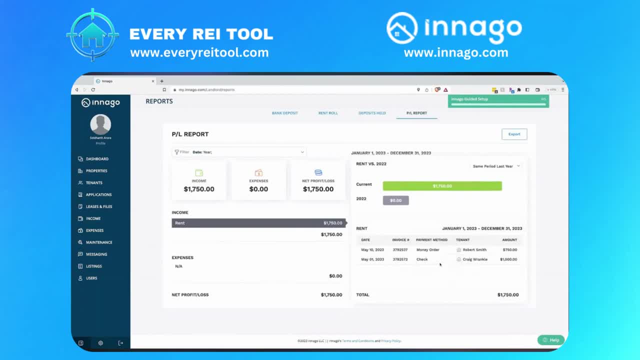 payments that are that kind of comprise this category. so if i had late fees here, if i had, whatever else it may be, it's all going to appear here. all the expenses appear here, giving you a nice sense of the health of the business. you can filter to a specific property. 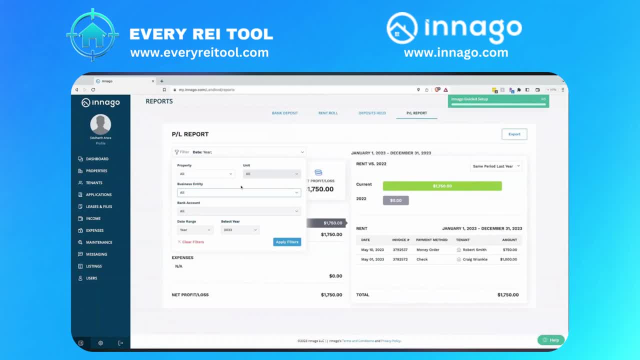 a specific business entity if you have multiple llcs to manage your portfolio. um, so yeah, it's really easy to get kind of the data. that's that we believe to be most relevant for you as somebody investing in managing day-to-day, but again, it's not going to be the 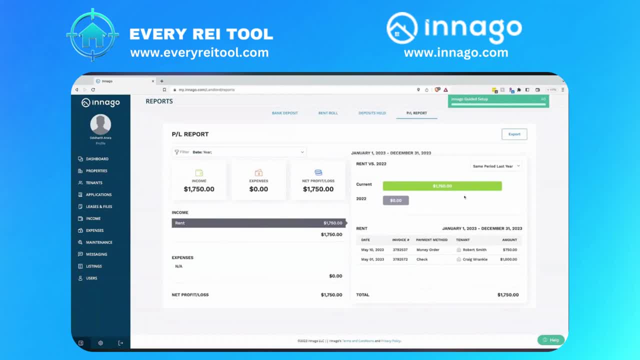 full-end back-end accounting stuff? no, no. robust software, yeah, no, of course not. but at the very least, like you say, if you can export what you need to give a competent cpa and they come back saying: you know pretty much, you know, i've got what i need to do my job, then good enough, right, especially if 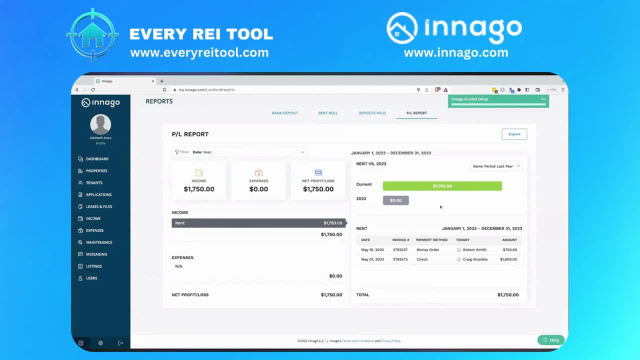 it's this clean and this easy. i love it exactly. you know we talk a lot about it because in the early days we said, hey, should should we be offering you know a full like general ledger style accounting, should are we competing with quickbooks here and, i think, a lot of property. 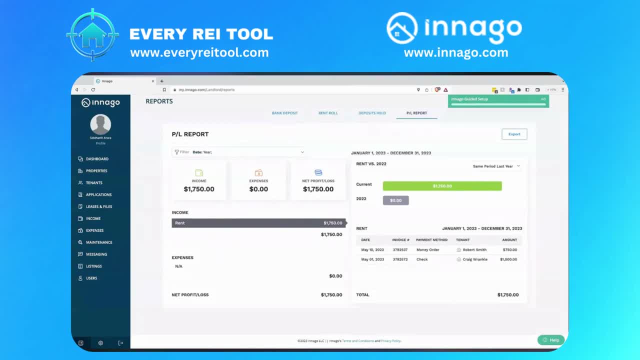 management software has made the decision to, yes, compete in that way, to offer that full-on, and what we kind of felt was that for most landlords, especially diy landlords, their day-to-day management software is going to be a little bit more of a distraction, and it's it adds the most. 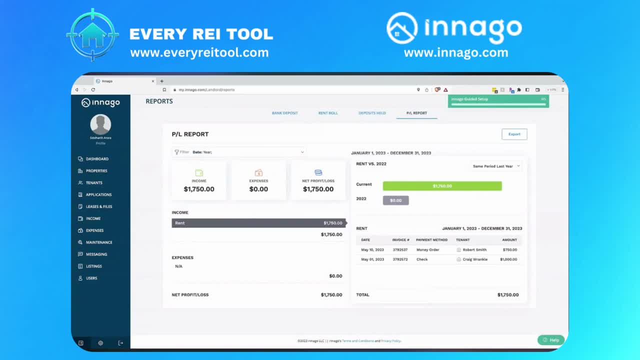 complexity to the software of anything else. um, so we said, hey, let other software that's that's built to do that, do that if you need it. we actually integrate with quickbooks. we are working on integrations, additional integrations with like xero, um, net suites, uh, a few others to to try to. 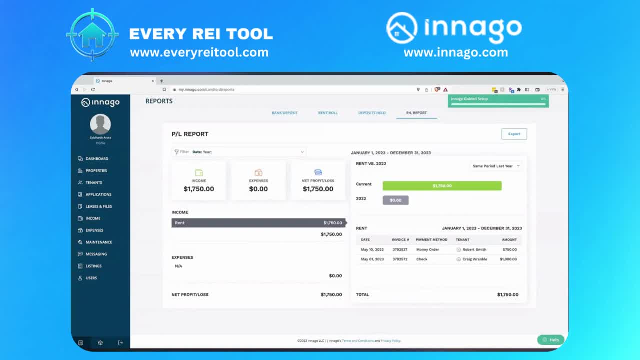 offer that for those landlords that need something a little more robust. but again, our focus is just on what's your actual problem. it's managing the tenants, it's managing collection. it's managing really really good and not distract with a lot of, you know, accounting tools that aren't quite as 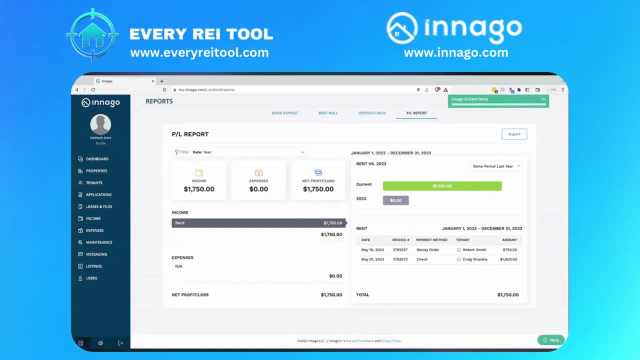 critical for the day-to-day stuff. yeah, totally. i was about to ask you because you did mention integrations earlier and it sounds like you're working on some of those integrations in the first place. so that's great. yep, absolutely, um, so, yeah, so the the financial reporting piece, you know we 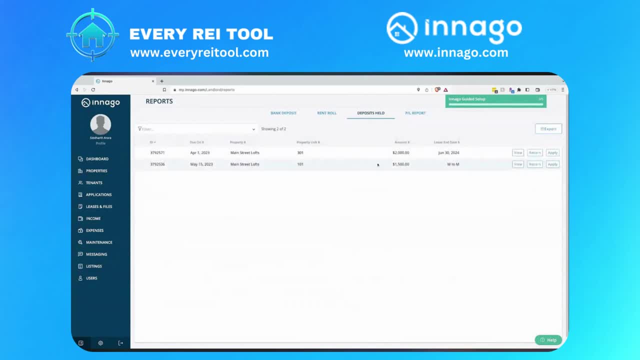 also have deposits held reports. so this is where you can track security deposits. um they are a liability, so they're not going to show up on the p? l. you can return them. um you can manage your rent roll from here. um you can manage the actual bank deposits that are coming in from inago, uh, if we're sending you funds electronically. so 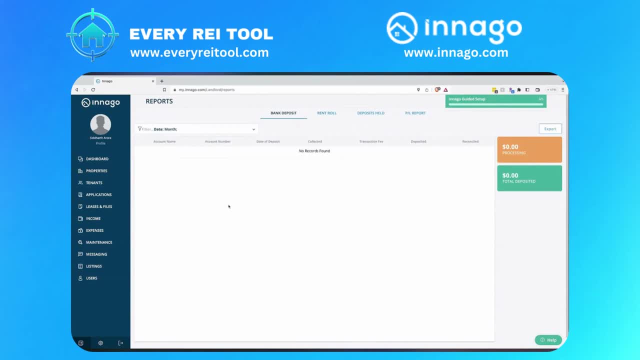 that you can reconcile that. um. so there are a handful of reports that you know are kind of the essential ones for you and they're nice and clean and easy to uh to interact with there, awesome, um. a couple other features just really quickly. um, like you mentioned, we have expense. 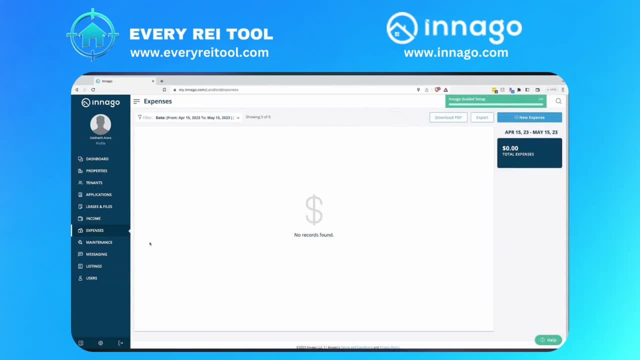 management. it's pretty straightforward, you know. you can enter those expenses, you can record them, you can take pictures of receipts, all that good stuff we are. we don't currently offer the ability to automatically pull in expenses, although we are currently working on it. uh, we're working with. 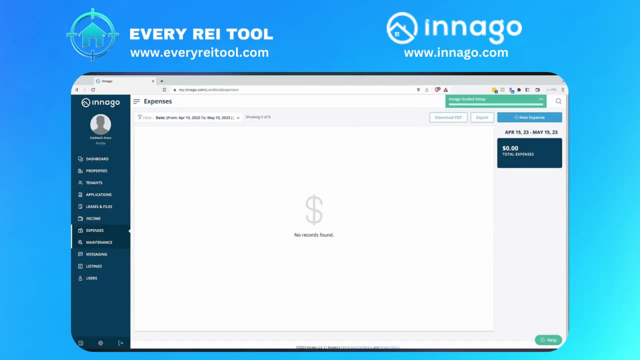 plaid on that. um, we're kind of the big name in that space, so that should be coming in the not too distant future, which would be a great plus for landlords. we offer maintenance ticketing and management. um, again, a pretty straightforward maintenance system. you can create those tickets. 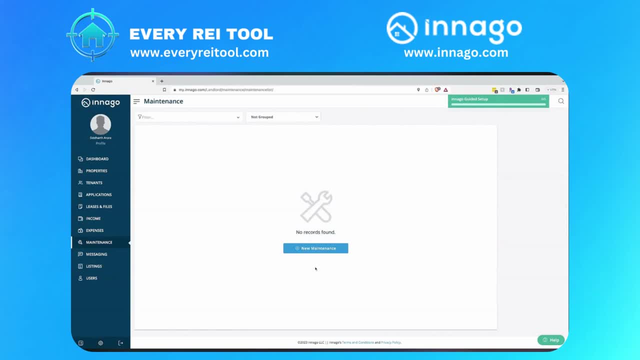 um, you can manage them, communicate back and forth with your tenants. it's possible, as i mentioned, to add sub users that have access to maintenance. so if it's just a maintenance person that you work with or a handyman that you work with, it's also possible to really easily forward a. 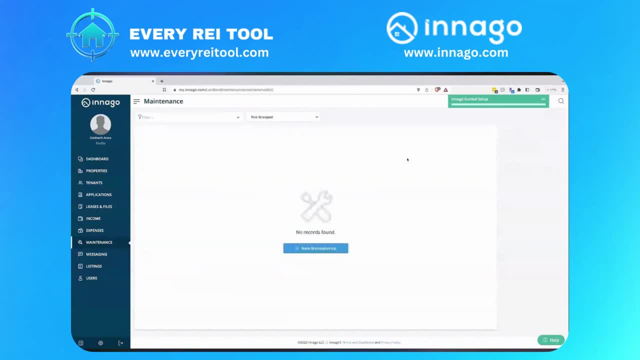 ticket and all the details, including the pictures and videos and descriptions etc. to somebody. so if there's somebody outside of your organization that you want to give access to a maintenance ticket that's coming in to help with it, it's really easy to do that in anago. 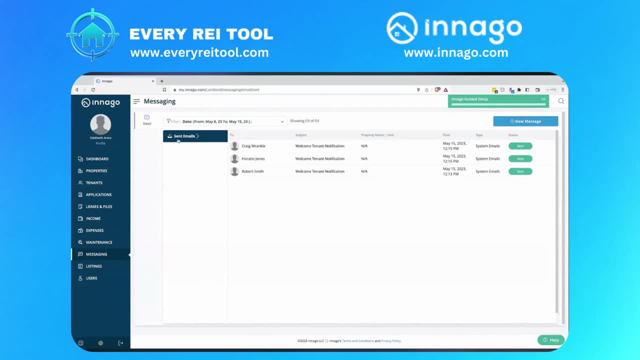 we offer the ability to email your tenants, and we actually have a feature that's coming out, i think next week- that allows you to chat back and forth with your tenants, so we're really excited about that. you'll see that right here below the email option: uh, coming soon. and then, finally, we 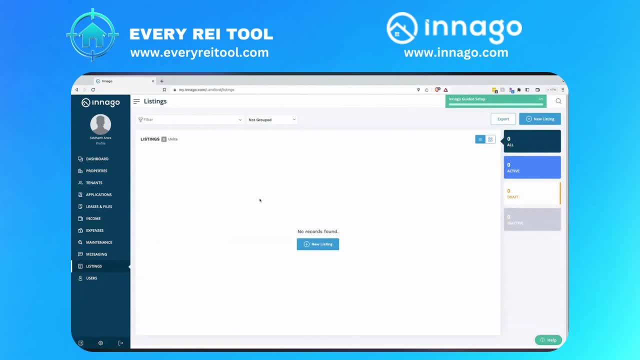 have a listing of your tenants, so if you have a tenant that you want to give access to, you can send them your mortgage credit and you can see how it's been developed. it's very easy to send them down and we're going to offer a listing, as much as you can, of all the tenants in the 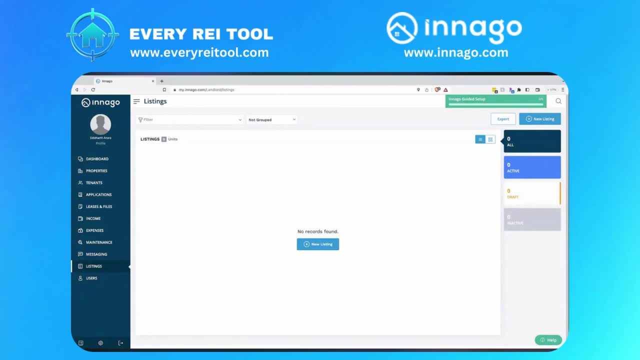 area and you know we are a major contract singing in here and you know we do our our retail network. so if you want to send a rental deal in, we do a lot of rate servicing and that's where we're finishing the retail deals. uh, and you know we're going to look for insurers and 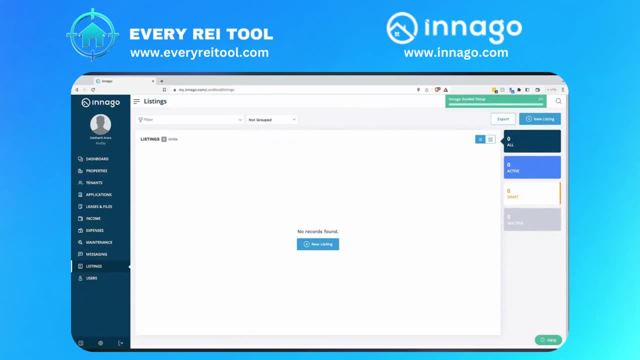 zone directors and people that can help you with that as well as we do other listings. so we do syndicate to uh realtorcom network, the zumper network, the rental source network and the zillow as what we're seeing here. but what's the experience like uh for the tenant, is it? 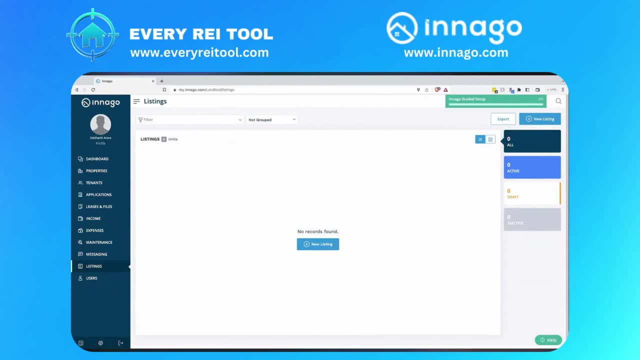 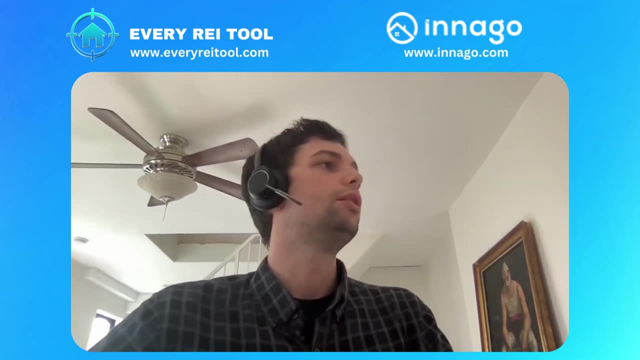 you know, very similar to what we're seeing here. yeah, that's a great question. let me pull up a tenant account really quickly. i should be able to do that, um, and i'll show you, and i can show you both the mobile site and the- uh, it's a lot of people that you know watch these or listen to. 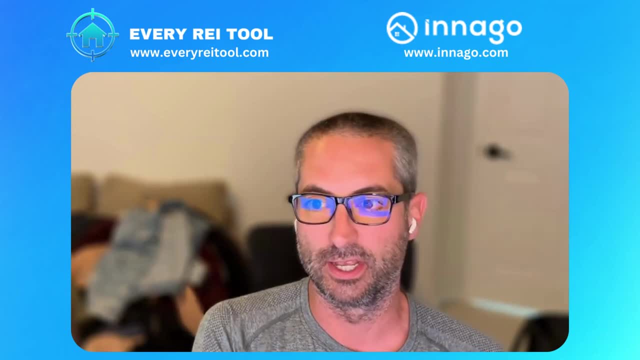 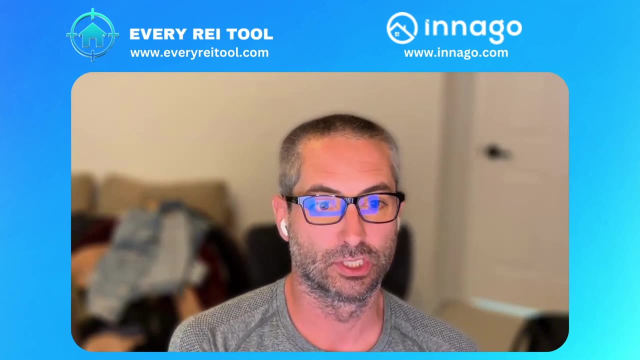 these right. they're interested in the full experience and they want to know not only what it is for themselves- kind of you know quote selfishly- but also what you know. how easy is this for you know the tenant right and some questions that i get often when you know reviewing. 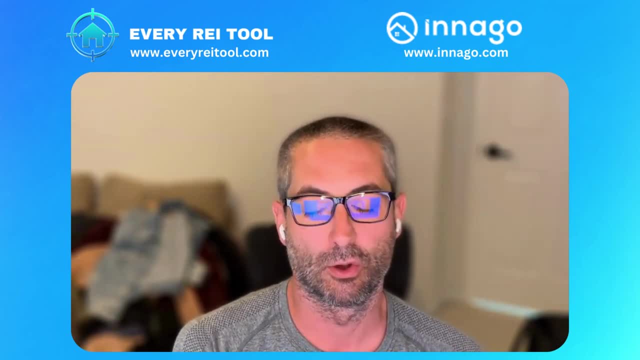 these is- and more and more so today- is like, for example, does it not go report to the credit bureaus when rents are, you know, paid paid on time and whatnot, because that's becoming more and more important to renters? yeah, that's a great question. we do. we currently work with trans union and it's 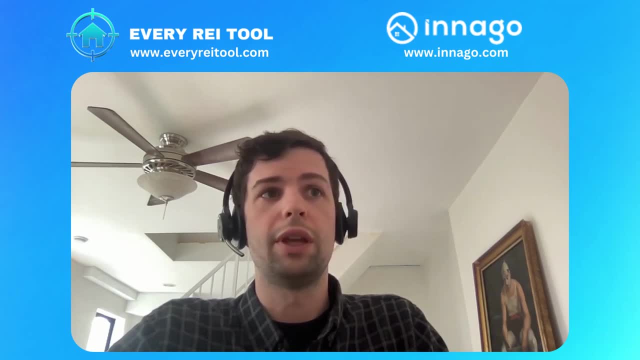 a totally free service. there's no additional cost to tenants to get that reported. they can just enroll and they get that advantage, which i agree is a really important thing these days, um. so yeah, we do offer that we also. i'm glad you brought up the tenant piece, because 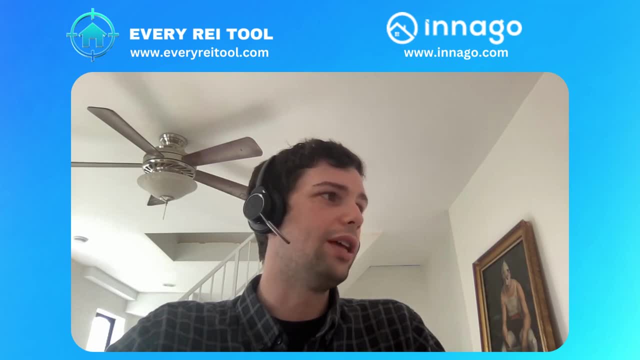 that's something we talk a lot about. you know, we kind of think of it like um. you know, amazon thinks of the shopping cart: right, nobody's bought anything until they've paid, right. so the easier you make that process of paying, the easier you make that process of interacting with you as a 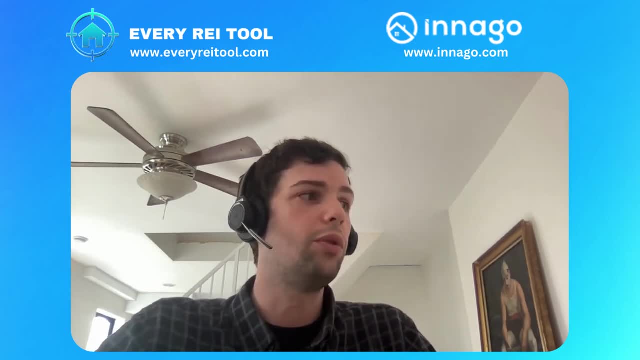 landlord, um, the better your collection is going to go. so it's so important that you have an easy interface for your tenants to interact with and i think historically that has been a challenge and problem for a lot of property management software. where they're just, you know, they're signing a contract and charging the 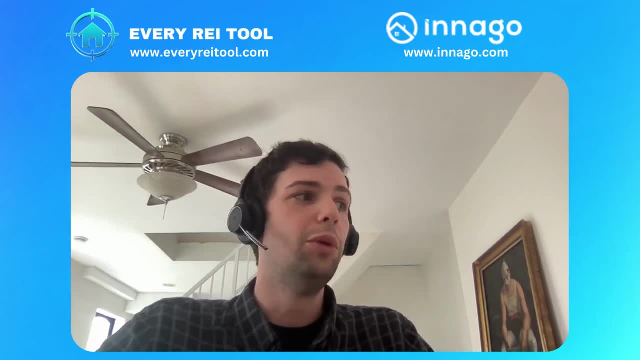 landlord a monthly fee so they don't really care about the tenant experience. but because of the nature of our system, where it's totally free to use and they're just kind of engaging with it at will, it's critical that our tenants have a great experience. so we really prioritize that and do our. 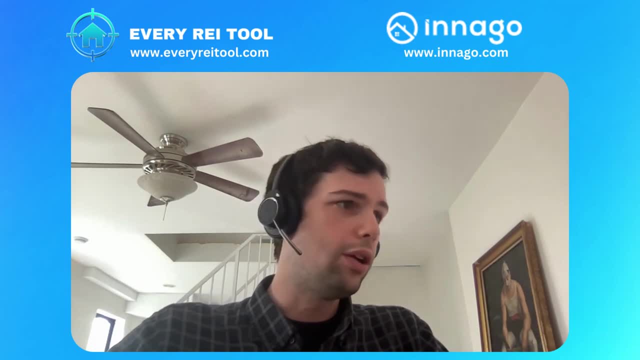 best to uh to make sure it's super easy to use. so yeah, i have an account here um it. you know, bear with me on the data. it's just kind of older test account data again. but let me share my screen again and let me know when you can see it. 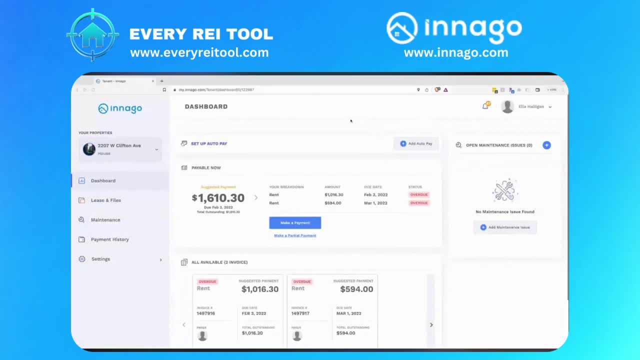 all set, okay, awesome. so this is ella's account now. she's a couple years overdue here, uh, so she's definitely in trouble. might not be renting there anymore, but you can see the breakdown of of the total amount that she owes um the total amount on each individual invoice. she can quickly and easily 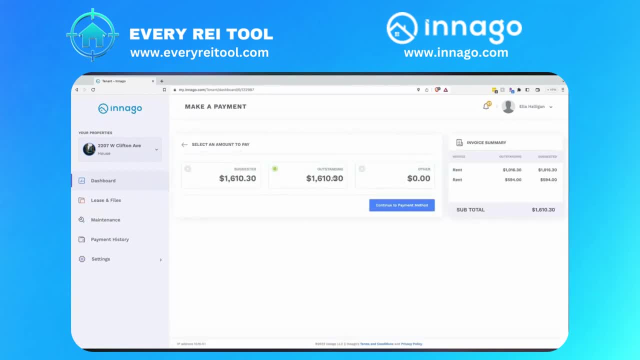 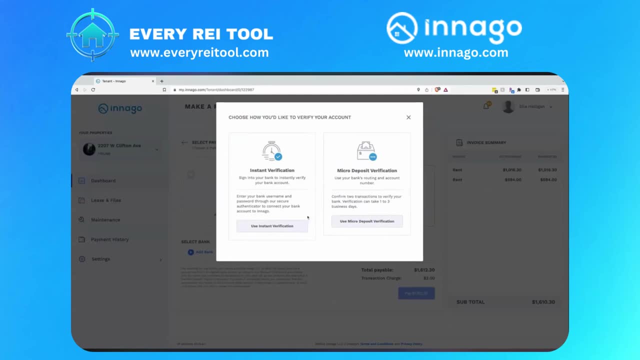 click to make a payment and choose how much she wants to pay. let's go with the outstanding amount. she can add her payment method and she can choose how much she wants to pay. and she can choose how much she wants to pay as needed here, so she can add a bank again. we work with plaid, so the bank. 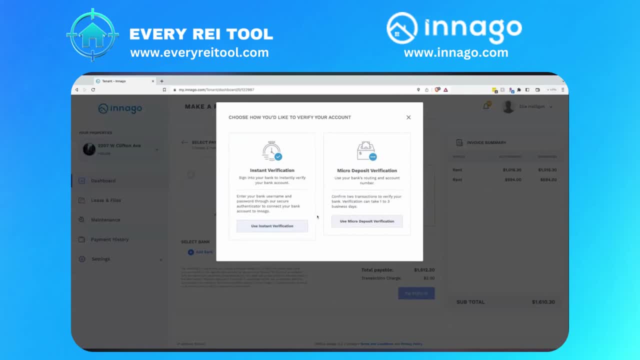 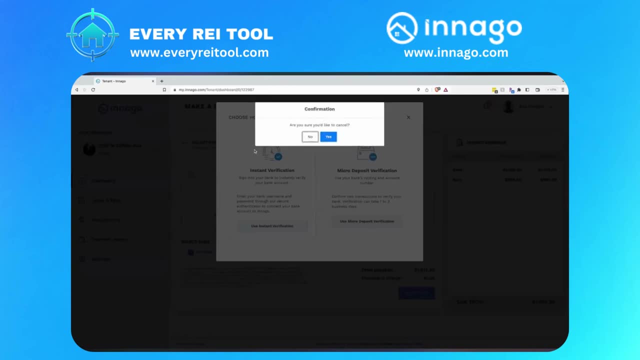 verification is super easy: you just connect right through to your bank offers tons of coverage. if they don't have a bank that connects that way, they can use the micro deposit version right. the tenant can sign up for autopay once they do have a payment source added to inago so that it 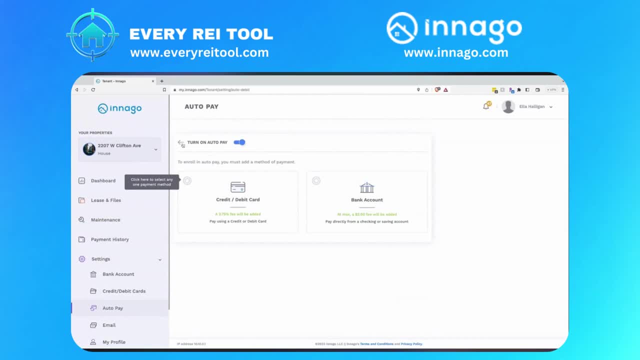 comes out of their month every or, excuse me, comes out of their account every month without any issue. so that's great when we we strongly prompt tenants into adopting that. um, if they have any documents uploaded, they can review them here. if there's a document that needs. 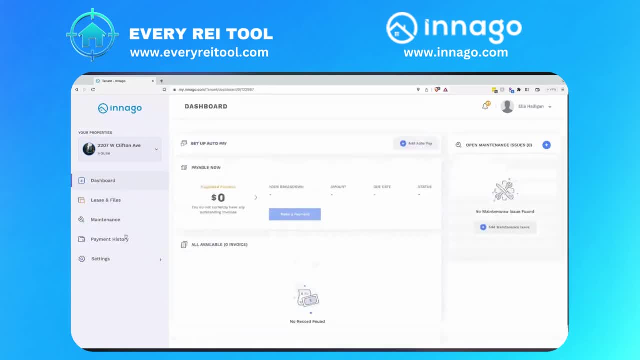 to be signed. they can review it here. they can submit maintenance tickets, which, again, i mentioned that they have the ability to upload. it looks like this landlord turned off maintenance for this particular tenant, but they have the ability to upload pictures and video, um, add a description etc. categorize it all. yeah, i imagine they'll typically do that from, like the mobile device. 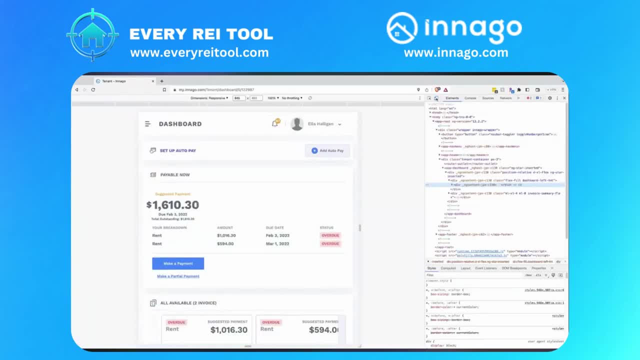 right. much easier to walk around and take a picture of their leaking sink and there you go. that's exactly right, and here i'll just show you kind of what it looks like. yeah, so in the mobile app looks almost identical to this, but this is the web mobile view: really clean, really simple. 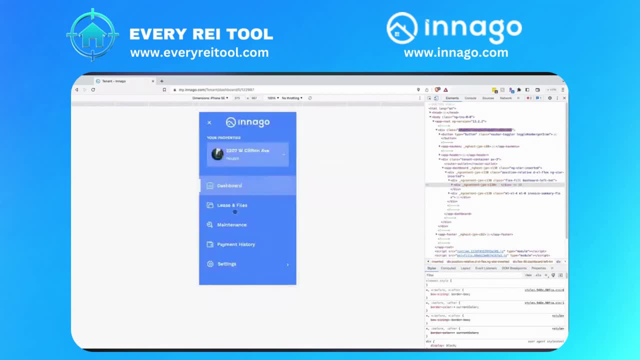 easy to use, interface, easy to interact with for the tenants. um so typically tenants have very little trouble. usually they're more tech savvy than the rest of us, so they don't have any issues figuring out how to how to pay their rents, uh, when they need to. very cool. anything else we should see? 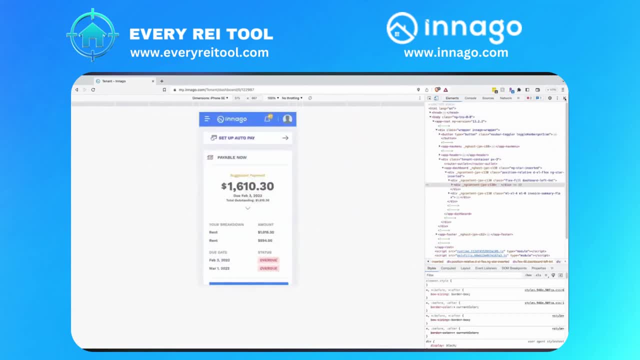 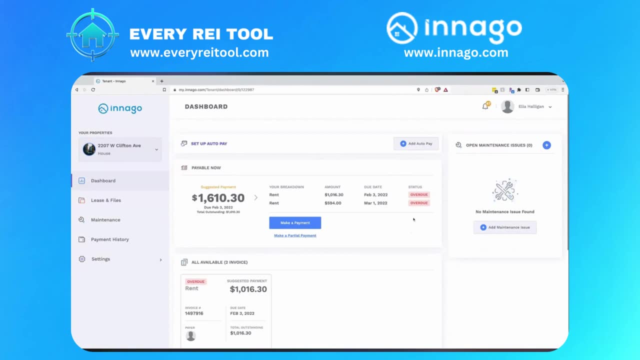 in inago. it is so cool, clean, it seems so easy to use. i think i might have to start managing some of our properties myself so that i could just use this myself, love it. yeah, no, no, i think we covered, uh, most everything. i mean we're we're constantly working to improve inago. i mentioned a couple features. 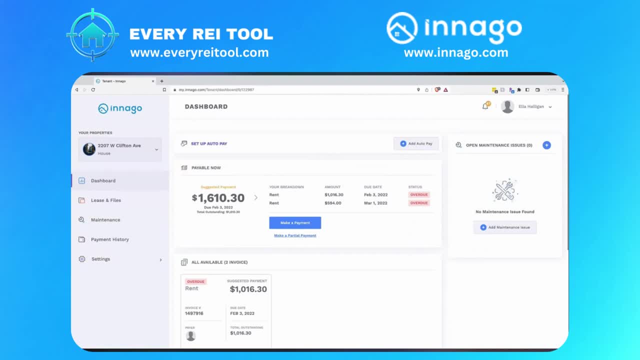 that are coming out here soon, like the chat. what are you most excited about coming up? honestly, it is the chat feature. i just think that, as so like for landlords, you want to be able to communicate effectively with your tenants. it's such an important part of managing your rent. 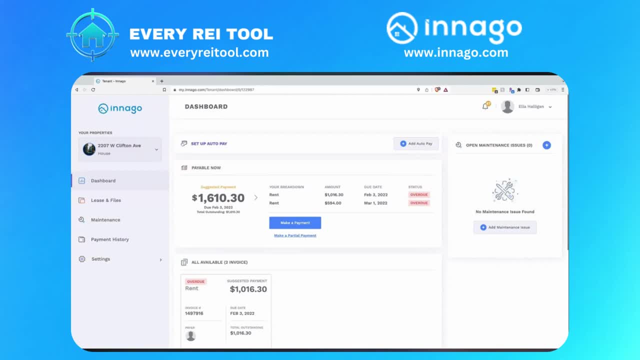 but you also want to separate them from your life. right, but so often i feel obligated to share my personal phone number with my eight units that we have, and i hate getting texts. you know i never save their name in it because i'm like i don't want to have my. you know their name cluttering. 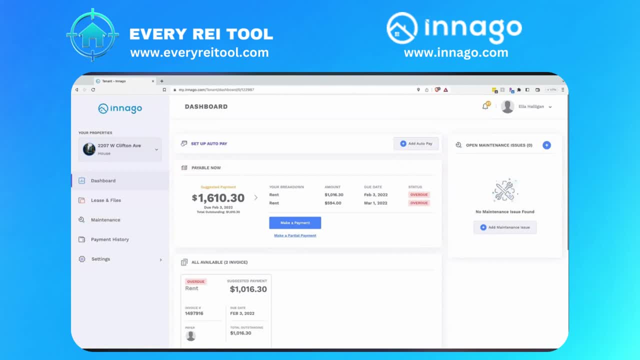 up my contacts and so to be able to just chat and communicate directly through inago, uh, really seamlessly, is something that i'm personally excited to use as a user of inago. so that's a big one that's coming up here. um, i'm trying to think other big ones. the expenses is going to be. 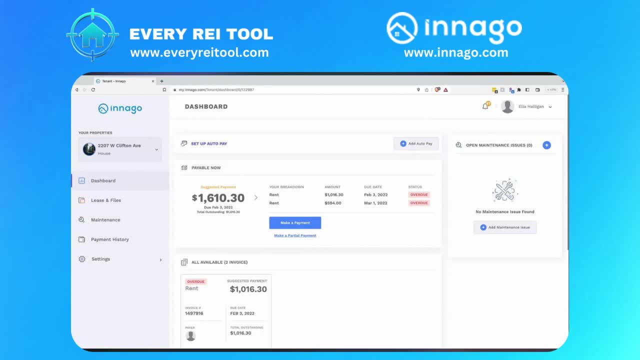 a great feature. i'm trying to think other big ones. the expenses is going to be a great feature. um, there's some some like funds, return stuff that we're doing, some vendor management stuff, so there's some exciting things on the road map. yeah, very exciting. super clean, seems to be super simple. 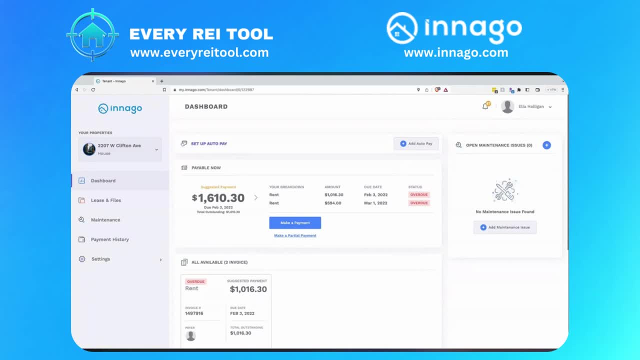 love it. um, this is inago dave. thank you so much for your time. i don't want to take any more of it. we'll leave, of course, uh, all the information um in the show notes here, but you can always go to every reitoolcom: slash, go, slash, inago, and you'll get there, or go straight to inagocom. 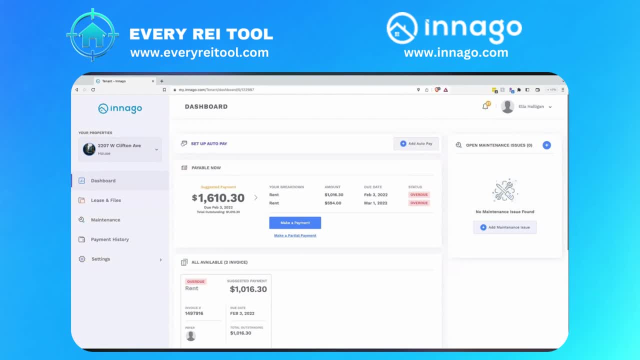 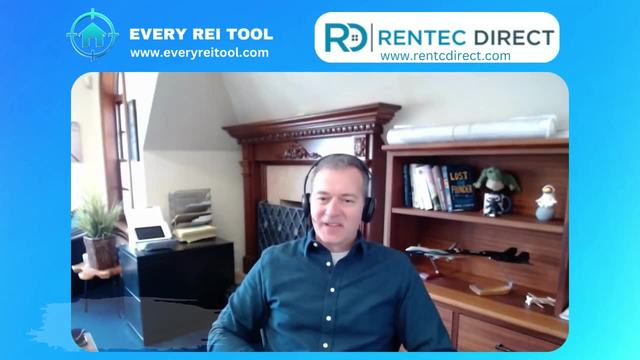 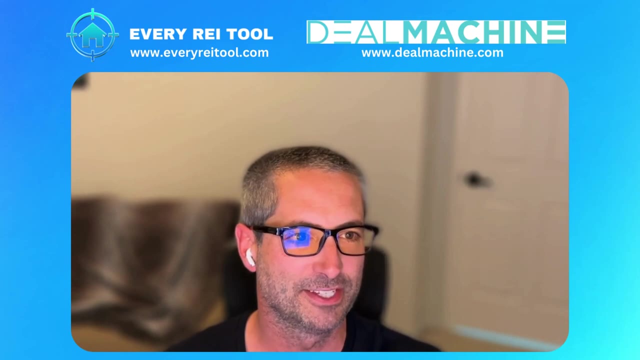 and with that dave, thank you so much for your time today, really appreciate it and i look forward to having you back on. we got all these new features for sure. thanks so much, nathan. perfect. how about yourself doing well? thank you very much. we have both uh same initials, so we're gonna keep things simple and hopefully not. 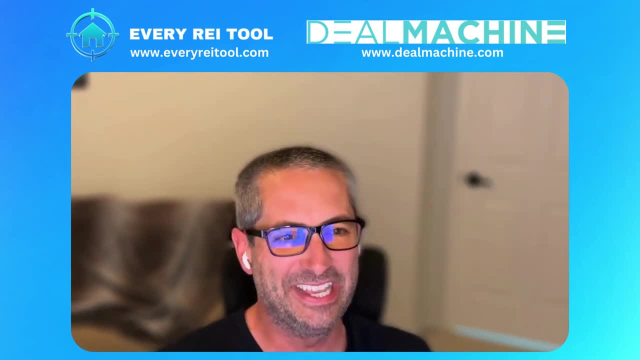 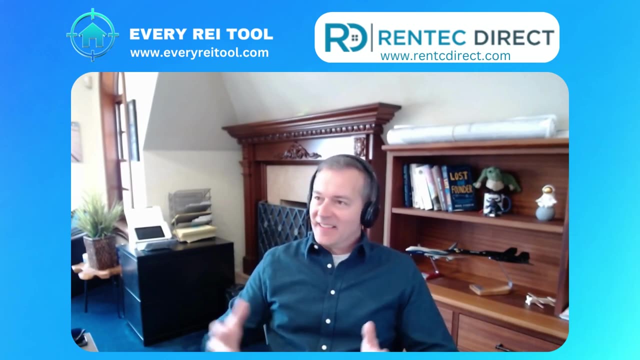 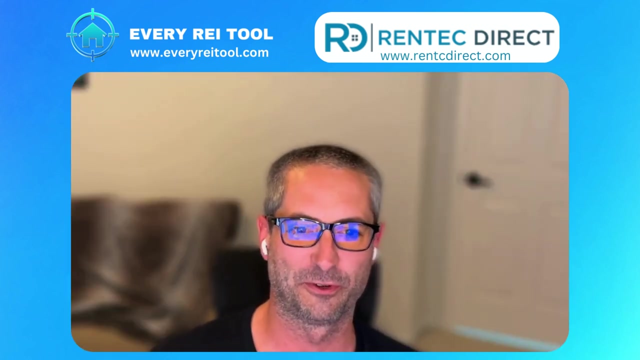 get our names mixed up, um, in any case, so you are with red tech direct, nathan, what's your role over there? uh, i'm the founder of the company and now i get to do the- uh, the presidential ceo over here. now i love it. so what's the quick, like elevator pitch for what rentech direct is? 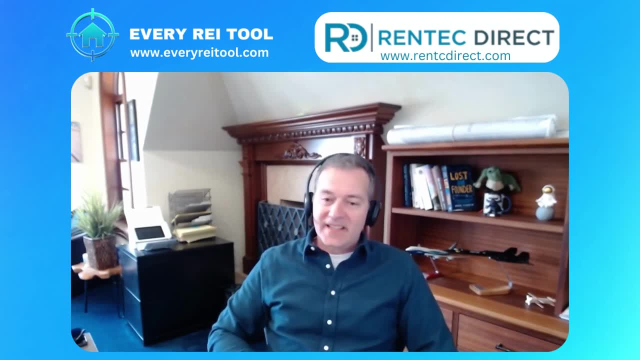 yeah, rentech is an application for property managers and landlords. it's, uh, designed to pretty much take all your tasks, automate anything that is possible to automate, make your life as easy as possible, while providing a really cool tool for you to be able to interact with your 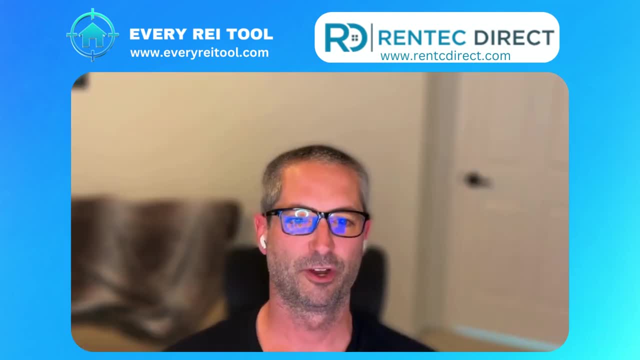 tenants or your owners? if you're a property manager, very, very cool, and who would you say this product is typically for? because there's a lot of you know property managers and property management, you know software out there. i'm curious who your, your preferred or target audience is. for this you bet. well, we love working with all private landlords, whether you have one unit or 2 000 units. most of them end up in the 20 to 200 unit range. we love working with that size. we also work with property managers up to about 2500 units. that's that's kind of our sweet spot is 20 startups. 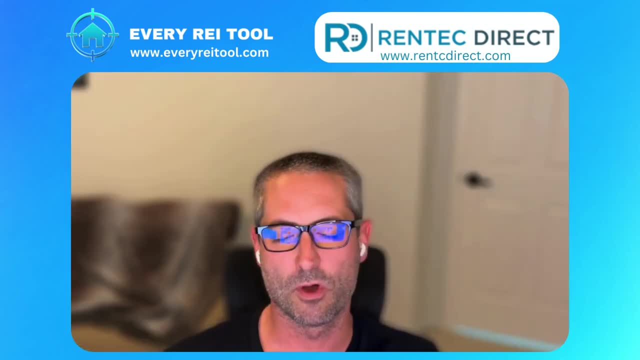 up to 2500. got it, and would you say there's anyone that this tool is not for? so maybe those that have more than 2500 units, but i don't know if there's something a bit. you know more specific about where and when this tool is not suited. yeah, i'd say the huge corporate property management firms. 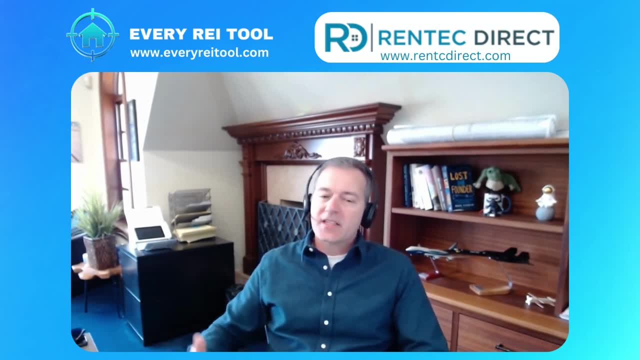 that have tens of thousands to hundreds of thousands of units. they just need more than we're putting in the software which might include, you know, payroll, corporate accounting and stuff like that. it just gets way too complex when you add all that stuff into the system and our system. 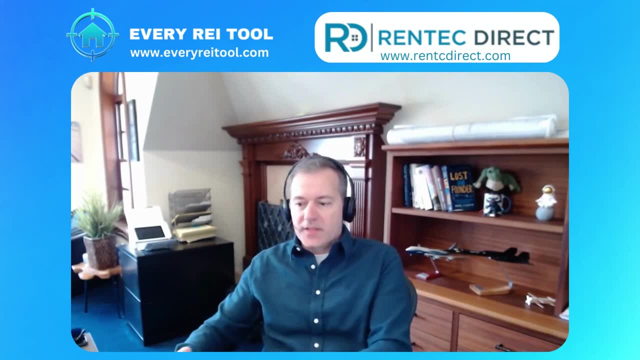 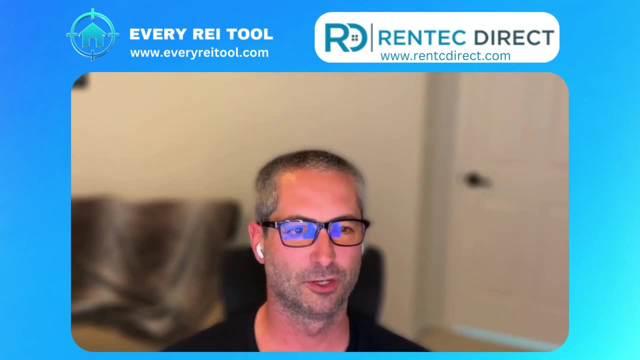 was really designed to be quick to start, easy to use and easy to you know. have your staff on. very cool. maybe that's the perfect segue for one of my favorite questions here. but what do you feel rentek does better than other systems out there? yeah, we kill it on customer. 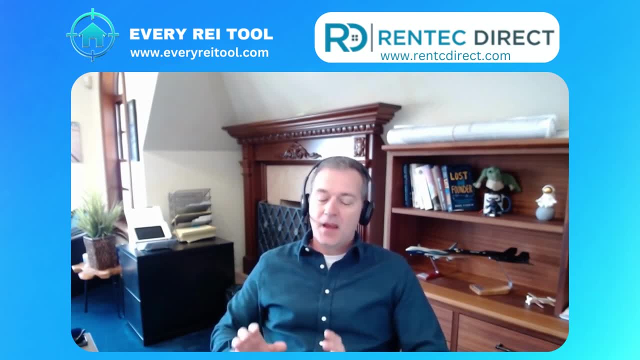 service. we've got a us-based support team. most of them actually take in property management certification courses, so they not only know our software really well, but they know the industry really well, and so they're going to be able to help not just with our software but every unique. 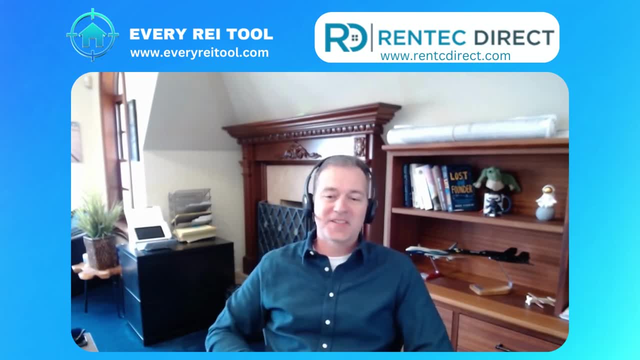 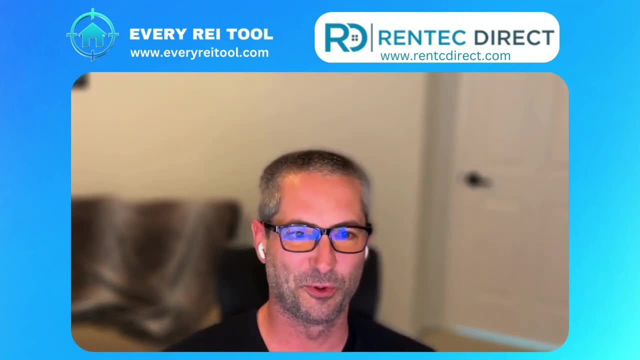 circumstance that tends to come up when you're talking about a property management certification. the property managers- oh very cool, that's awesome customer service. not a lot of people you know brag about that, so i'm glad to hear that you know. awesome quality, perfect. um, and before we hop over, 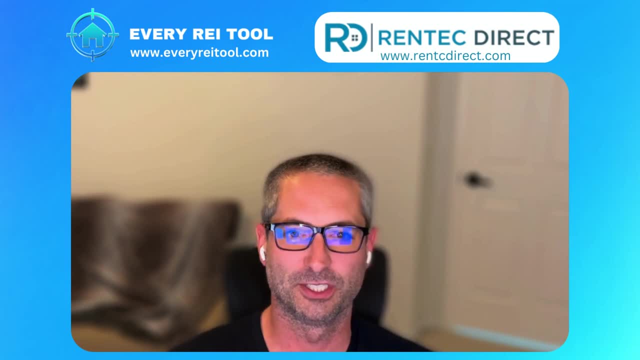 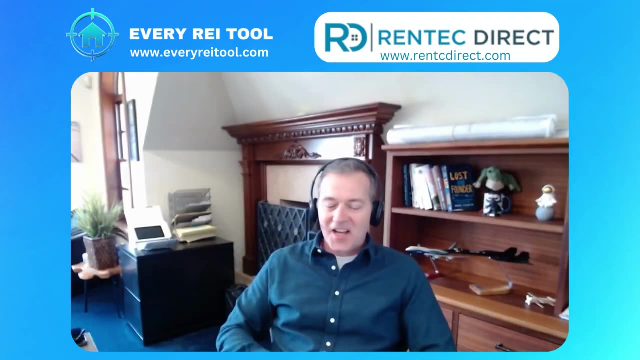 to the, the demo here of the product itself. last question i'd like to ask is: what is the price point for this tool, because everybody needs to know how much it's going to cost. right, you betcha? we? we charge about 1.10 per unit and we have a 45 minimum, and that includes your merchant account. and all the tools that we supply are built-ins. there's no extra fees. you're going to be able to do all your bank transfers from your tenants to your account for all the online payments. that's all included. electronic signatures is included. work orders is included. it's all in there. 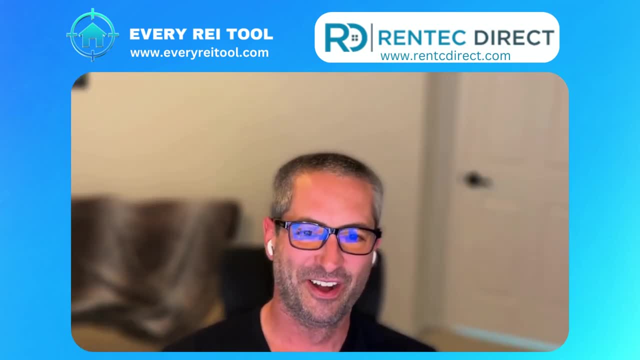 a buck ten. that's pretty cheap. if you ask me, i love it. all right, let's uh. so let's hop into. uh, what everybody's been waiting for here. if you don't mind, could you share your screen, maybe, and take us through a little bit of what this uh. 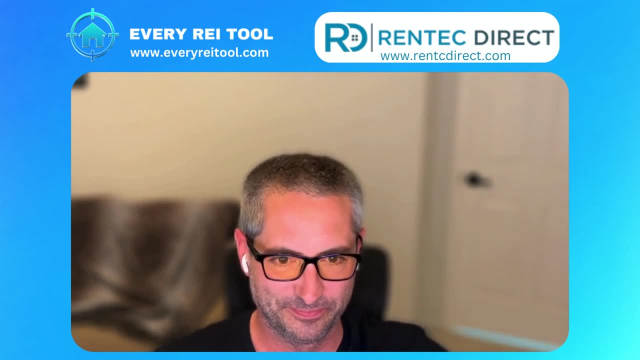 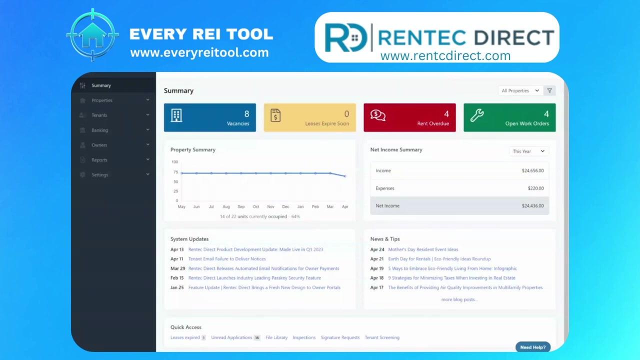 product can do for tenants, absolutely, and landlords, i should say, not just the tenants, perfect, i can see your screen. let's see what we got here. okay, so i'm on the uh pc, so this is a web-based application. you can ask access anywhere you have an internet. access works equally well on your phone, via the app or via web browser. 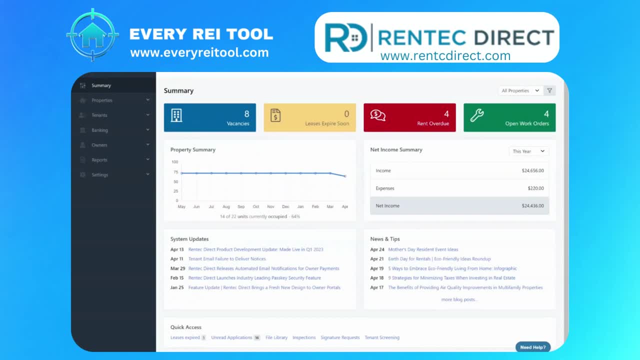 and we're looking at the management interface that's designed for the landlord or the property owner. now you can also use a website like mindset to get a little bit more information about what's going on. i'm just going to show you a couple of things. uh, there's so much more here. 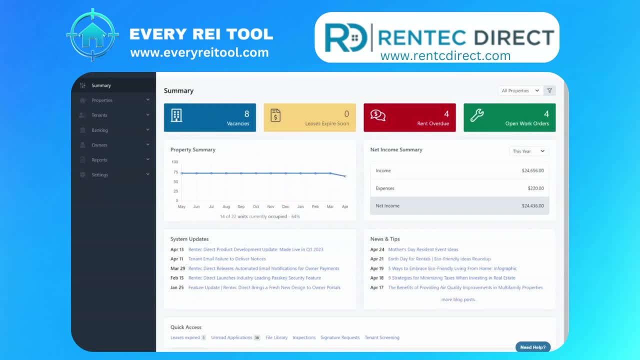 there's an app called appopropertiescom where you can go into a lot of the things that they say to you about you know the property and i'm gonna give you a little bit of a preview here- where they actually manage the relationship with all the tenants, record the income, post the property. 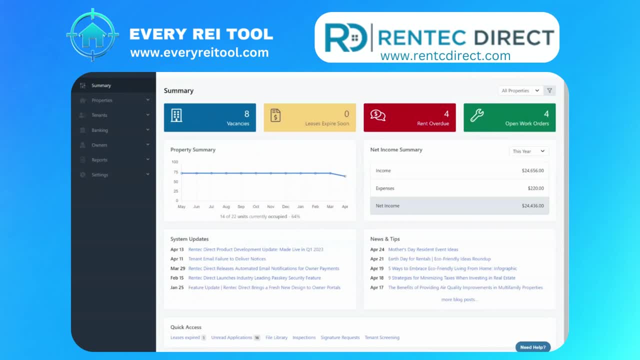 expenses, all that good stuff. there's also applications for the tenant and if you're a property manager, I'm just going to show you some of the highlights about how I use the system, and I'm already logged into just my demo account here and what you get is just a summary of what's going on with your company, and some of the things are highlighted, like: I've got four tenants that are rent overdue, I've got four open work orders and I have eight vacancies. 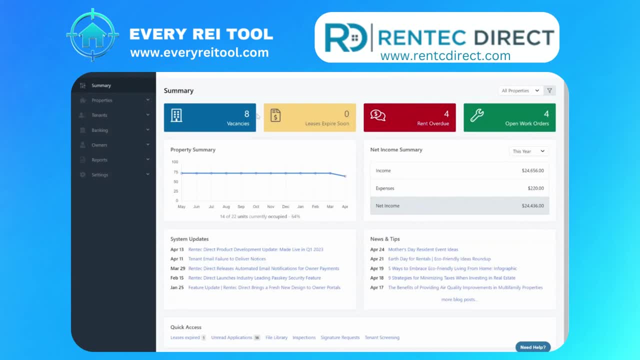 No one wants eight vacancies, right. But you can just go to any of these sections of the software by clicking on them. it'll zoom in. it'll show, for example, my four overdue tenants right here. they're seriously overdue, as you can tell from my demo account. 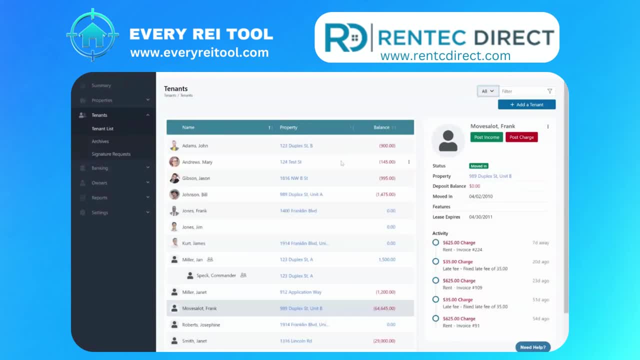 You can change the filter to whatever you need. here's some more realistic tenants, But what we're looking at right here is the tenant screen where you're going to manage, Add tenants, post income, post charges to those tenants and, like I mentioned before, we made the system just really easy. so if you're starting out as a landlord or you're a new employee at a property management company, the system is almost so intuitive that you can just get in here and you can figure it out just by with a few minutes, just clicking on one of these tenants. and let's just take- well, let's just take- John Adams and if we're going to post income for him, just a simple. 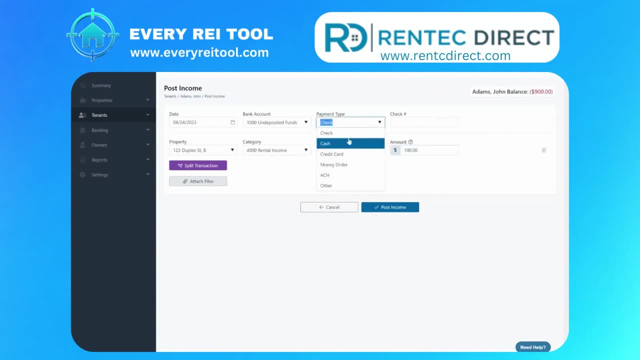 as that. you know we're going to take $100, it's a check. if it's ACH, you know it's going to automatically transfer those funds for him. but in this case I'll just post a $100 check. 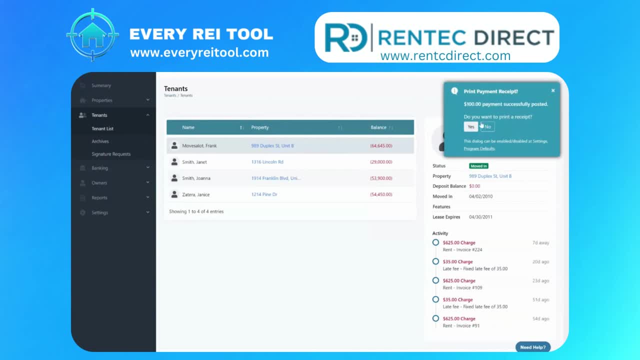 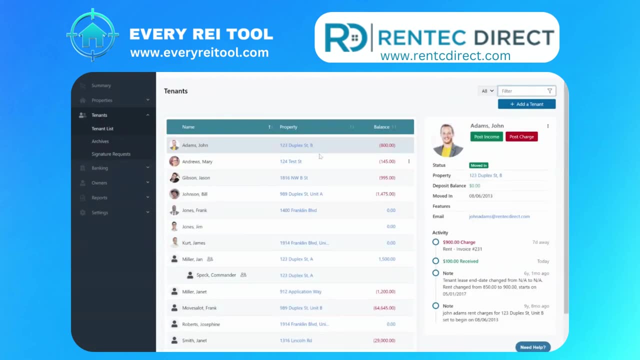 That's going to go back to our overdue tenants here, but it's going to let you print a receipt for him. and let me go back to my full tenant list here. and you know, John Adams now is only $800 overdue instead of $900 overdue. 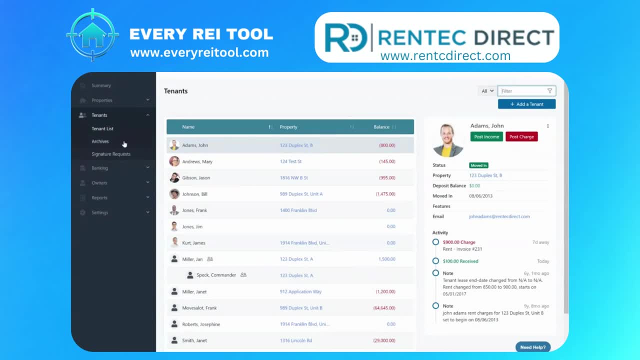 So I'll just blast through a few of these screens just because there's so many items. but you can see When we see here, we see add tenant. I'm just curious and sorry if you're going to jump into this, but when you add a tenant, is it just like adding an entry to this list of tenants or does it go through like the screening process as well, like tenant screening process? 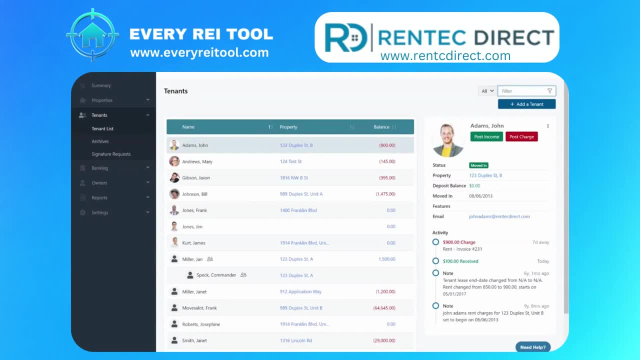 We have a full screening process and what that process would kind of look like it wouldn't be in that specific add tenant section, because what you would generally do in our system is you would list your property- which is another feature here- under properties. 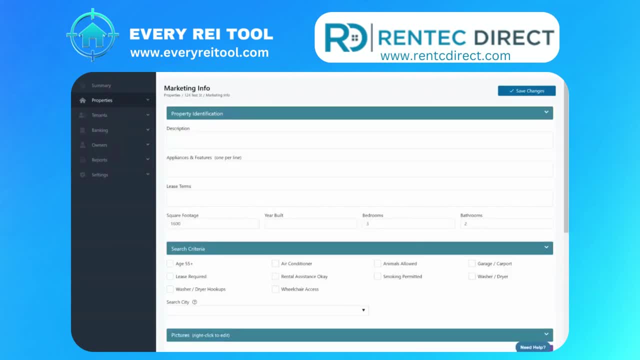 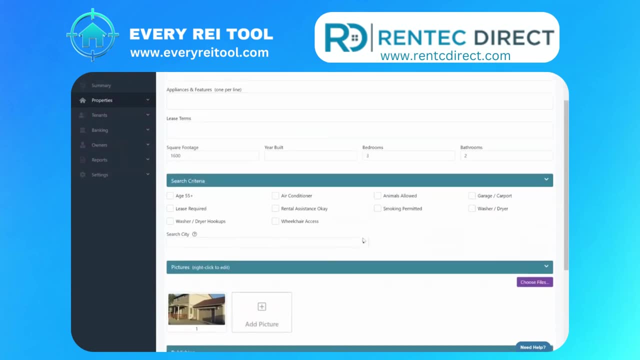 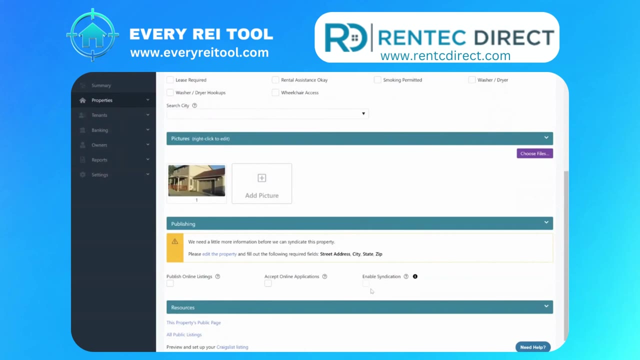 Let me actually just go to the marketing info on one of these. Pardon this, I wasn't planning on coming in here. it's all empty right now, but, as you can see, you can plug in all the information for the property, you can add pictures and then you can publish an online listing or you can syndicate it out to like 30 different sites. 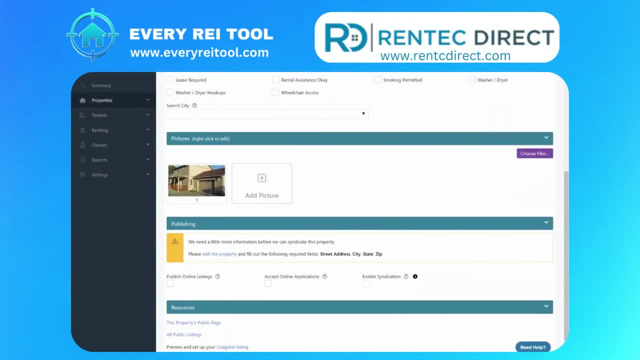 That way, you get the maximum exposure for your tenant. Now, when the tenant finds your listing, they come to the website that we're hosting for you. it shows all the pictures. it gives them a rental application link, which you can The tenant. 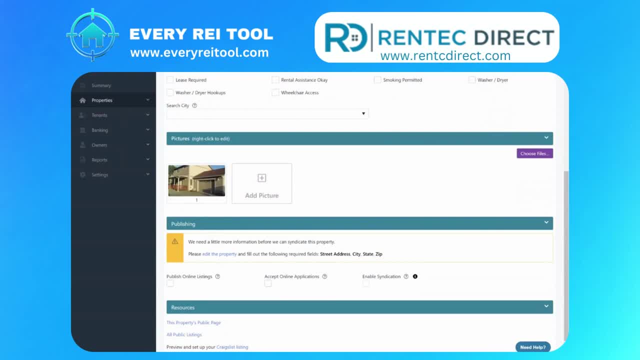 Can fill out all that information brings it into the system, in which case, yes, we will do credit, criminal and eviction screening. those are services that, since the tenant's already input all their information, all you have to do is click screen. it runs it through the system and these are all instant reports that usually come back in less than a minute. 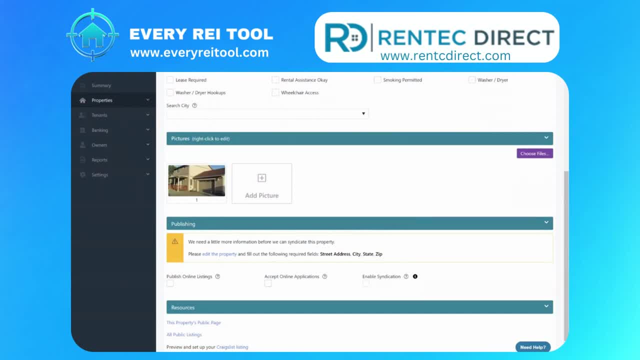 And then the publish online listing here. that goes to like your hosted version of this listing and if you syndicate, I'm assuming it goes to all the usual suspects. Absolutely yeah, It's going to get pushed to Zillow and rentalscom and realtorcom- there's a list of almost 30 sites that it'll go out to. 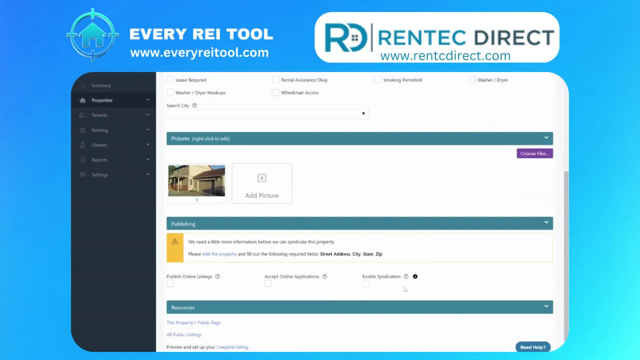 Awesome, Nice and easy. I love it. That's the idea it's. you know, it takes a long time to go to all those sites and publish this exact same information across every single one of them. You know, I mean, that takes, you know, five or 10 minutes a piece, whereas here you just put it in once you click the syndication button, we send it out immediately. you got tons of extra exposure for your vacancy. 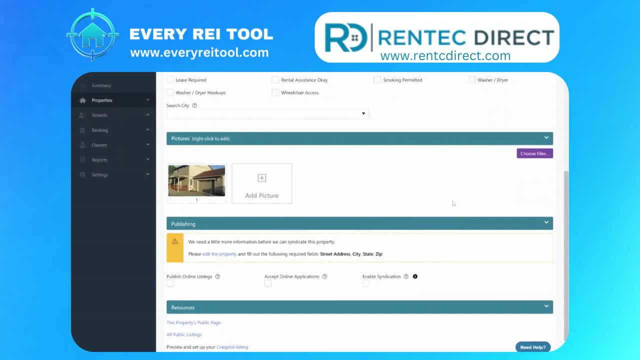 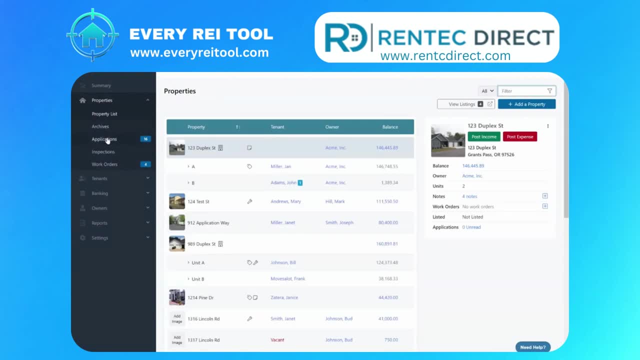 Because no one wants vacancies, Right? Nope, We want to get those things rented 100%. Yeah, you bet, Let's see. so in here you can. we were just talking about these applications. since we were talking about it, I'm going to just open it up and see if I got one here. 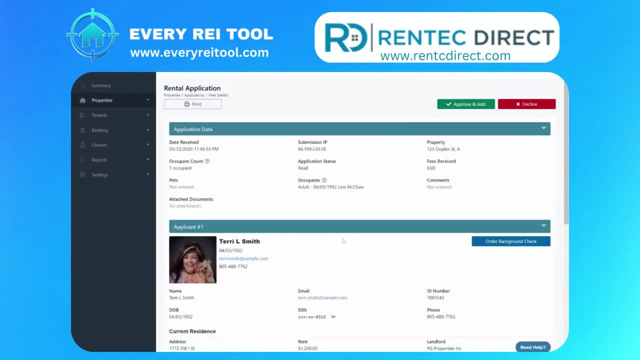 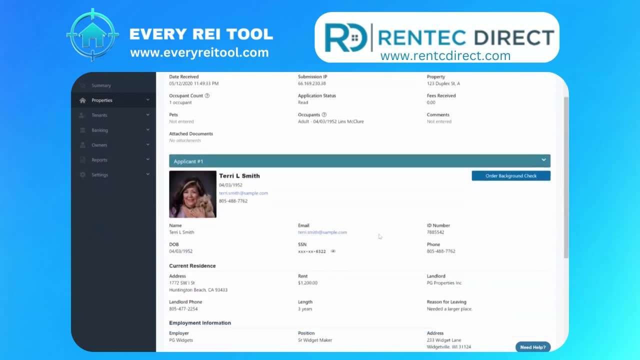 Lots of test data in here, but I'm going to go into this one. We were just talking about that. here's a sample application that's in here. It tells you all the information that the tenant might have included. Yep, If they have a social profile- public social profile- it's going to show up here. 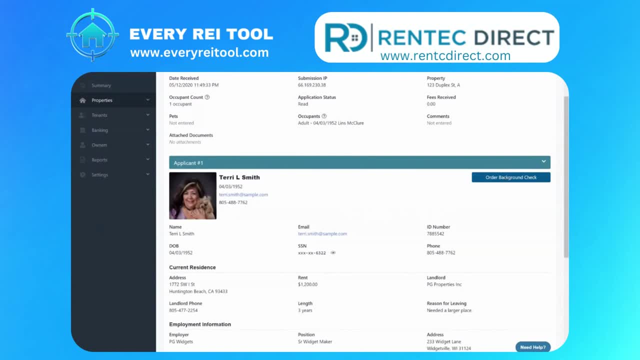 And then ordering background checks is just as simple as clicking that. It takes all their information and runs it through and gives you those, And there's no extra cost for the user. Background checks do cost. They're- oh goodness, the pricing on background checks. 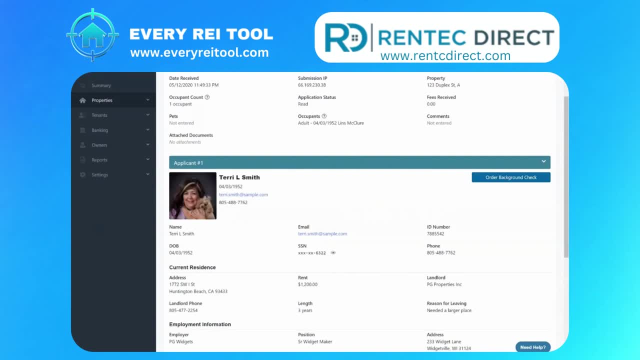 They're the standard fee. yeah, whatever it is, It's like 30 bucks or something They are. It's like it's: yeah, we go between 10 and 18.. We have a very wholesale deal. So if you want everything which is your credit, criminal and eviction, we charge $18 for that. 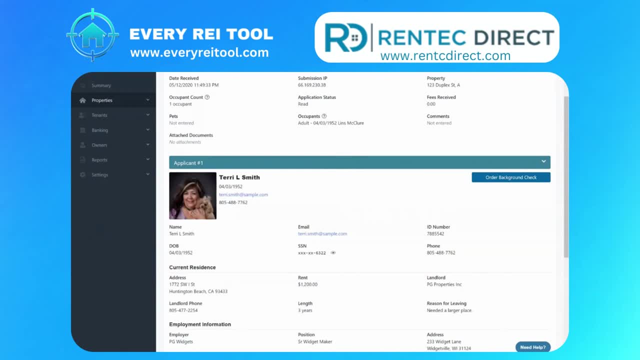 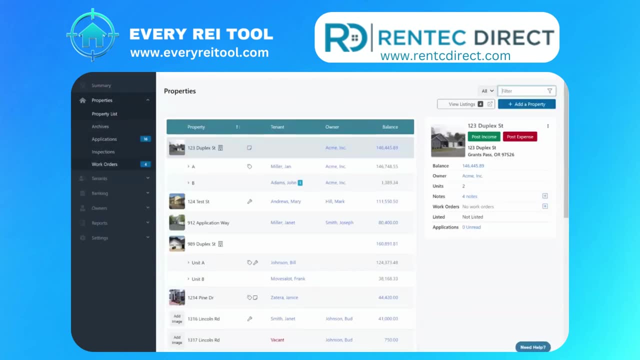 And that's those are for nationwide reports. Very good, Yeah, yeah, it's a great deal. Lots of people do use it. Oh, let's see, We also handle all the work order processing, So you got to keep track of what's wrong with your properties, where the problems are. 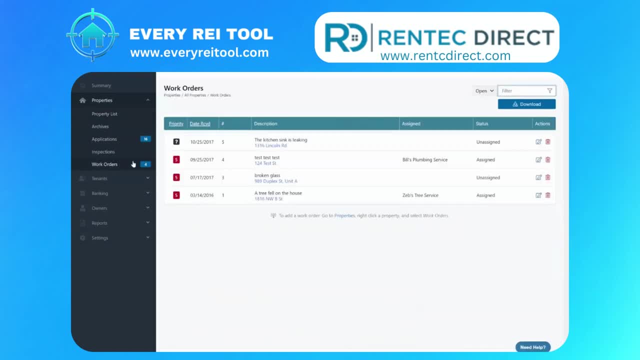 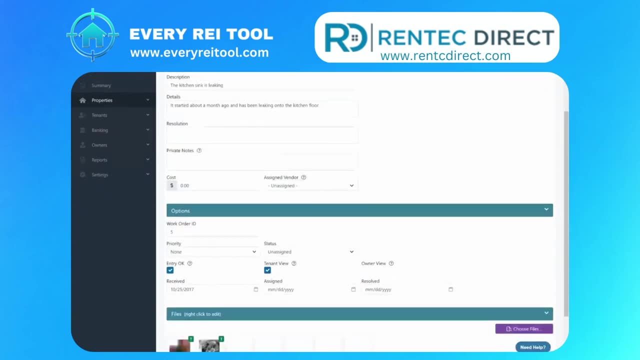 You can receive a work order. The tenant can also post a work order and it would show up in your screen here, just like this. You can go into that work order, edit it, assign it to a specific vendor- if you have a vendor that's going to be handling it. 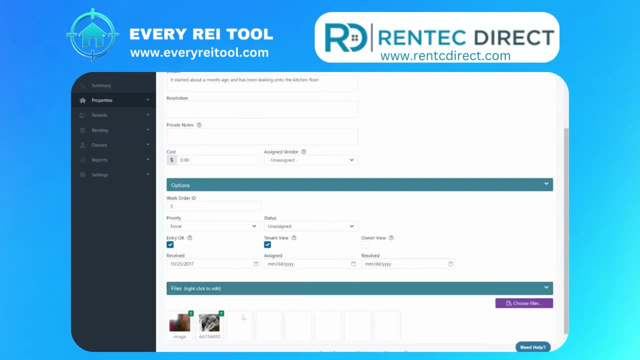 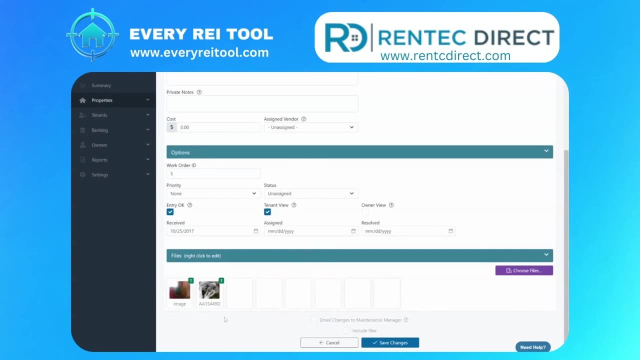 Post pictures. The tenant can also post pictures. As you can see in this one here down at the bottom of the screen, the tenant did post a couple pictures. I don't know what we're looking at there, but usually it's going to be a leaky sink, a rotten floor, something like that. 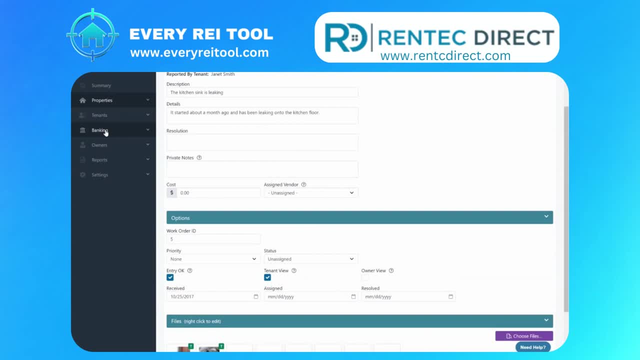 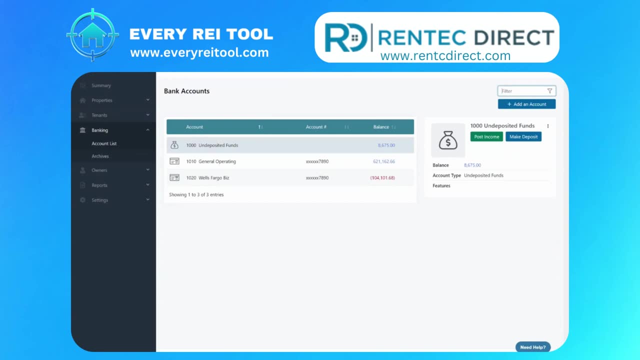 Of course. yeah, Let's see It also. one of the important aspects of property management, and especially for property managers, is making sure all the funds are in the right place. So we will do. yeah, you can plug in your bank accounts. 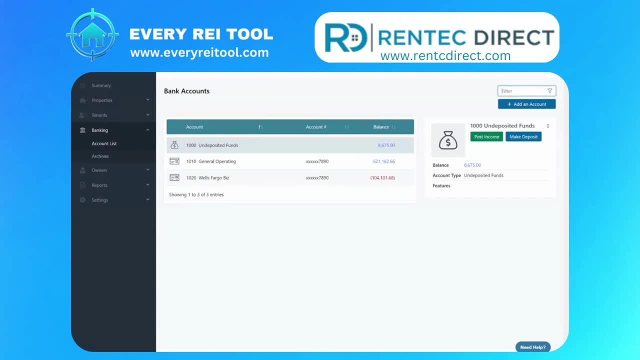 It's in here, and then you can even link your bank accounts So it'll sync, using a service called Plaid, a real common service that connects the bank accounts. It'll sync all your transactions on your actual bank ledger with the transactions in Rentech Direct. 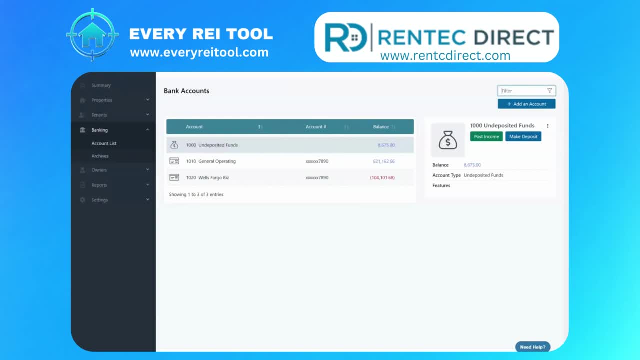 Just make sure nothing ever gets missed. If you have an expense that you forgot to record in Rentech, it's going to highlight it and say there's no matching record. That way you can plug it in there. Helps you keep your records straight. 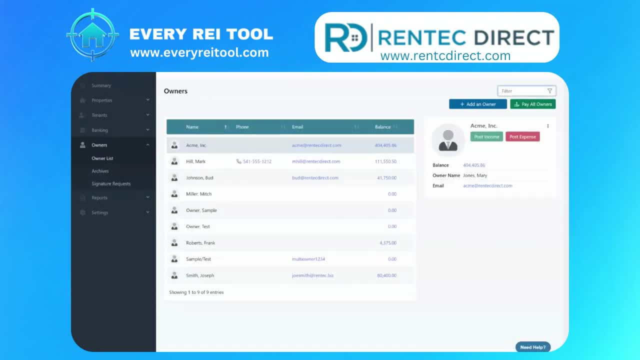 And sorry, did you say you offer banking solutions as well with this, or it's more connecting the banks to Rentech? Yeah, we don't do banking solutions ourself. Where we come in is doing those downloads, synchronizing the data from your, but then we also coordinate with your merchant account, which we set up for you. 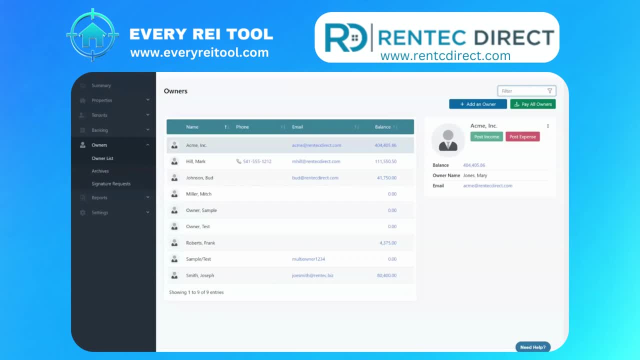 And that is included in the cost- to be able to transfer funds from tenants to your account Or, if you're a property manager, tenants to your account and then back out to the property owner? Yeah, I like to ask, Because some platforms do offer that as a service. 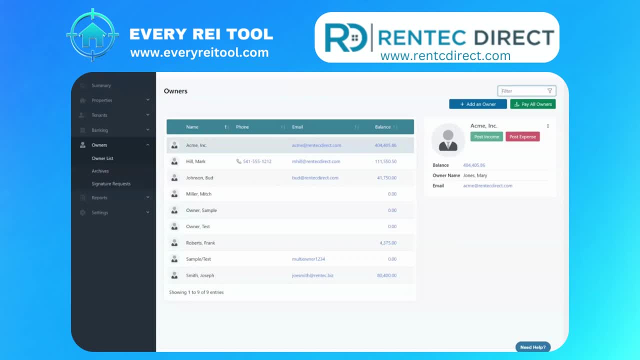 Um, so I just wanted to make sure I understood. Yeah, you bet. So in this case, this application is set up to work as the PM version of our software, which lets you also manage owners. So if you're a property manager, an important aspect of property management is maintaining those trust accounts and keeping every owner's funds absolutely separate from your own. 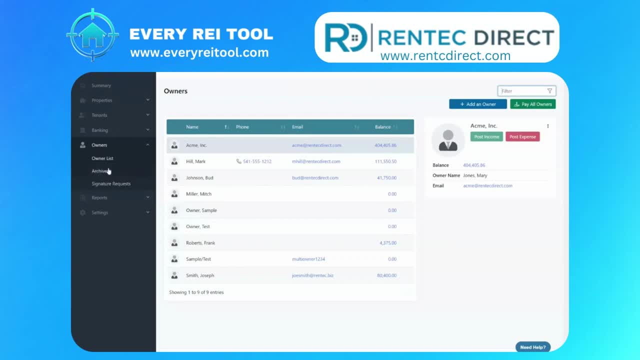 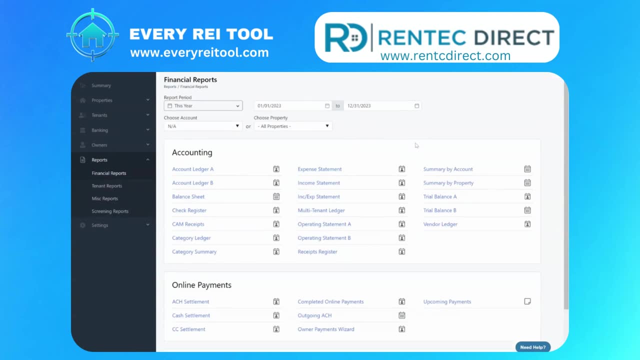 And, of course, separate from other owners. We take care of all that. Uh, it's all built into this System here, and then, um, and then a huge reporting engine- pretty much every report you could imagine that you need to be able to manage your- both your accounting, uh, and your properties. 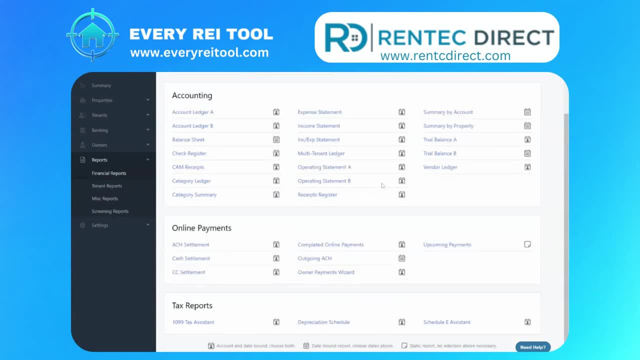 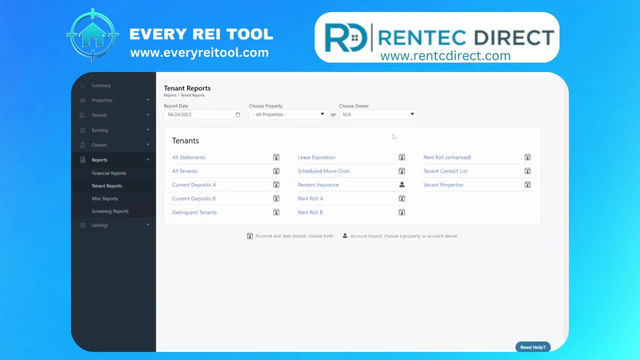 We've got a list of financial reports, which are all your basic reports. everything you would need, Um good list of tenant reports, your basic rent rolls, uh, tenant lists, you know, et cetera. Um a bunch of other miscellaneous reports, often related to property owners. 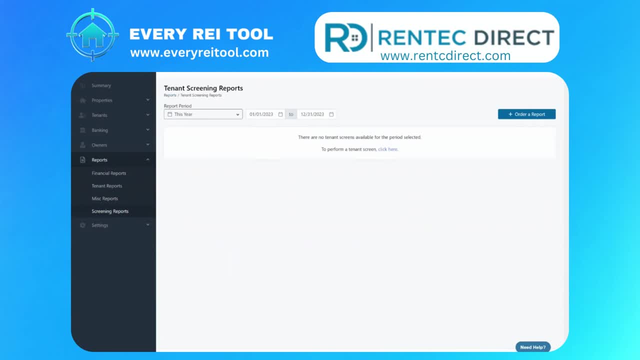 And uh, over here. Uh, I don't have any in this account, but here's where you would access all your tenant screening reports, So once you got one, you can historically go back in and check it out. Um, the other thing I'll probably pop in and show you here, cuz I know I'm just breezing over um a thousand features here in just a second. but uh, I'm gonna go into one of these, uh tenants. 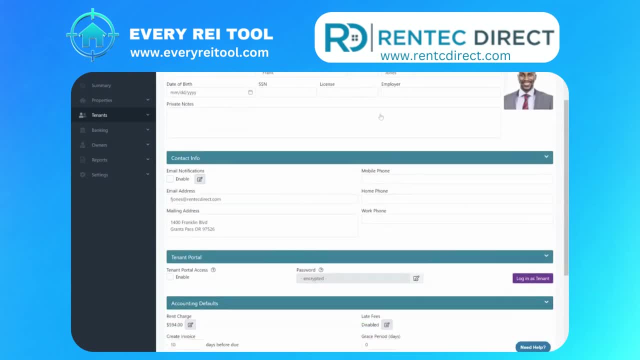 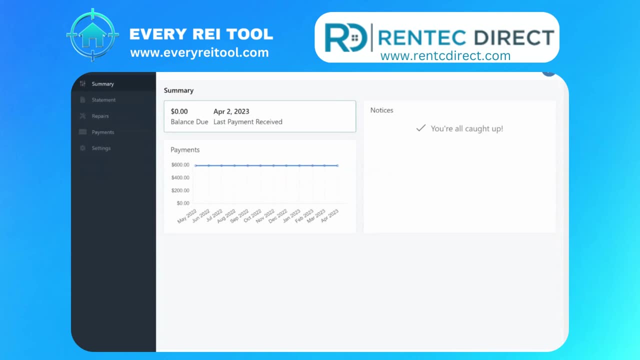 And I'm just gonna show you the tenant portal really quick. I'm gonna go ahead and log in, as this tenant um gives you now. Now we're looking at this On the desktop screen, uh, which everything's really big, um, almost all tenants using this on their phone via an app, um, or via a website. 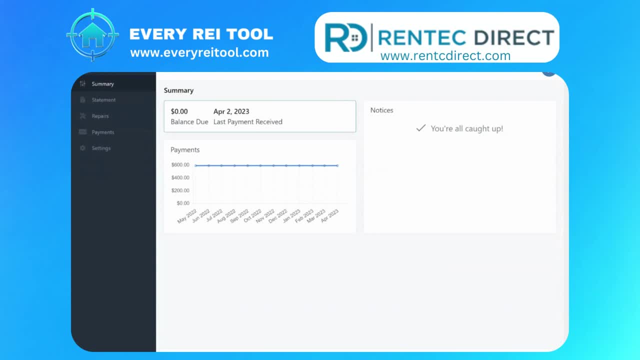 So all this stuff, you know, is going to be responsibly showing uh in the phone screen, Um, but one of the most important things, and one of the reasons so many landlords come to our service, is they want their tenants to be able to go and make payments online. 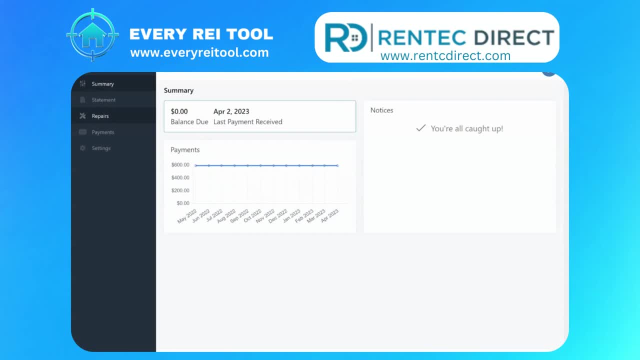 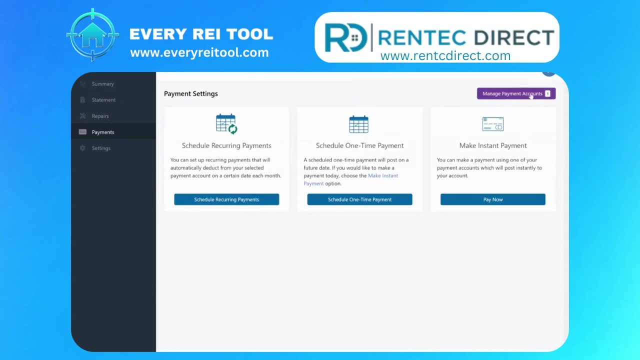 Uh, they wanna be able to schedule payments online, just for it to be easy for uh paying the rent. And uh, I just wanted to show you that here real quick. Uh, so this tenant already has a payment account that was set up in here earlier. 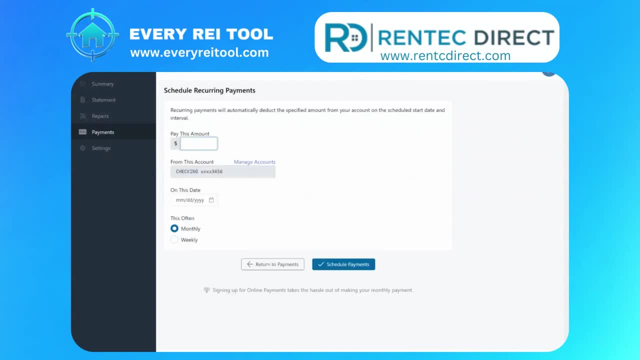 Um, but one of the popular things is just scheduling a recurring payment. Uh, this tenant has a thousand dollars rent per month. Uh, they want that rent, you know say, to come out on the fifth. um, every single month. they just schedule it. 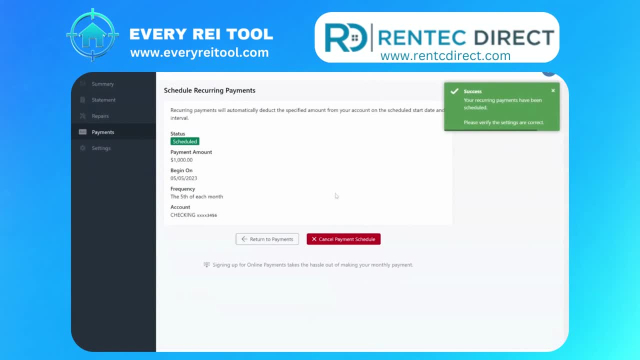 It's as simple as that. Now, every single uh month on the fifth, that thousand dollars is gonna be deducted from the tenant's account and and put into the property manager's account. they'll all get emails: Uh and uh. 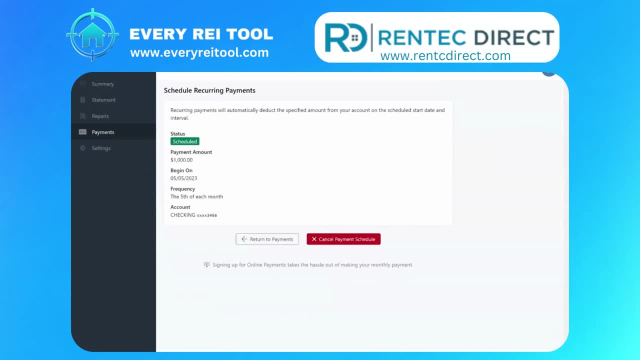 And the beauty of it is is all the accounting, all the reporting, everything is completely automatic, uh, that no one has to enter this payment. It just goes into that tenant's ledger, um, instantaneously. So just one of the one of the 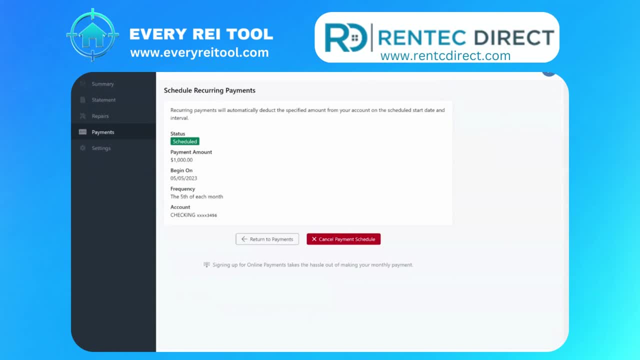 And this is the view where they would also, um, do like repair requests, maintenance requests, Absolutely, Uh, that would be right up here on under repairs And they could just report a new issue. and then that gets funneled to the right place- which is what you were showing us a minute ago- and gets logged. 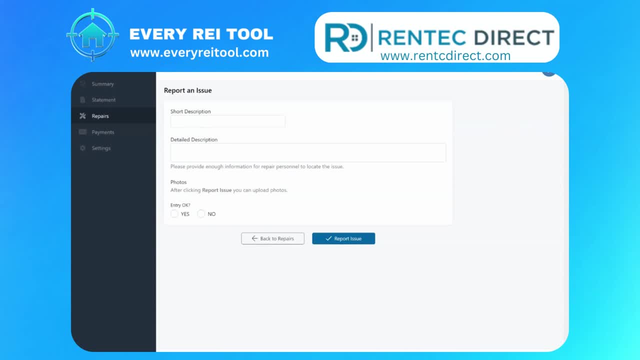 Absolutely, It'll show up right underneath the property. Uh, then, then the property manager can take care of it. If you're on the uh, if you're on a phone with a camera, it'll also give you the option to take pictures, uh, while you're submitting the maintenance request, so you can send the pictures right over to the landlord. 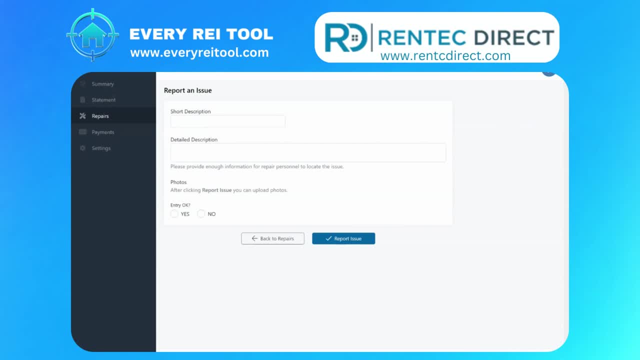 Awesome. So I'd love to ask you: is there anything else you would like to see? Cause I'm just kind of breezing over this and you know, not being a sales guy, I don't have actually a pitch, but uh, I'd love to show you anything that uh, 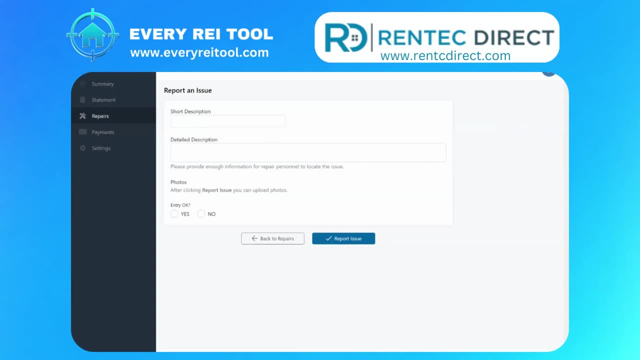 Well, I think maybe if we flip back to like the the owner or the property manager side, one thing That I've um seen come up a lot in like requests is actually there's two different things. They're both semi-related, but one is, like you know, accounting and transaction features. 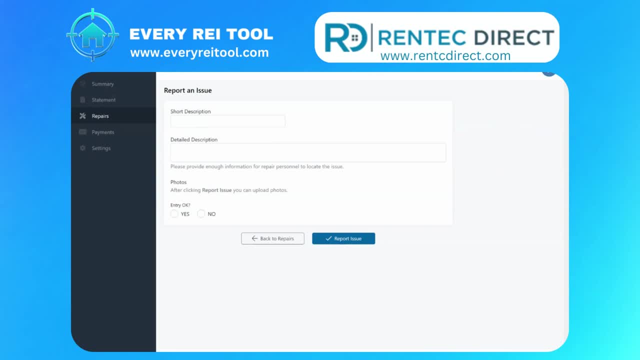 And I know we breezed through some of that. I don't know if there's a bit more we can see there. And then the other one is that we get asked: a lot is uh in the kind of reporting, uh aspects of these platforms is: what kind of reports do you have for, like tax purposes? 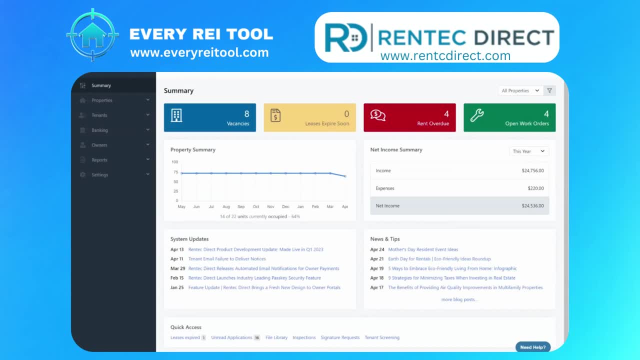 Cause I think we just packs past- sorry, tax day, Right, Um, and I don't know if there's anything specific you could show there, Cause those are two very commonly asked questions. Okay, And sorry, I uh I tuned out for a half a second while I was trying to log back into this here, but, uh, you wanted to see some. 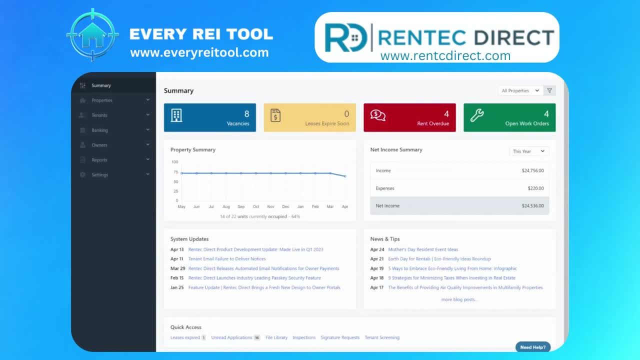 the first one is like, uh, like, um, transaction. you know accounting type, you know features. we breezed over those, So I wanted to see if we could go into a bit more detail there, Um, Like, just keeping track of transactions and things like that so that you can, you know, tag them appropriately to. you know, maintenance requests, CapEx, which. 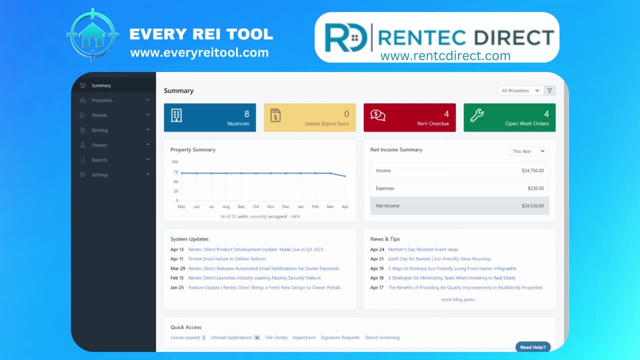 unit Which building things like that. Oh yeah, Okay, Yeah, Let's start there, Um, and let me go over here into our settings and, uh, show you all of our um chart of accounts here, just like in most accounting platforms. 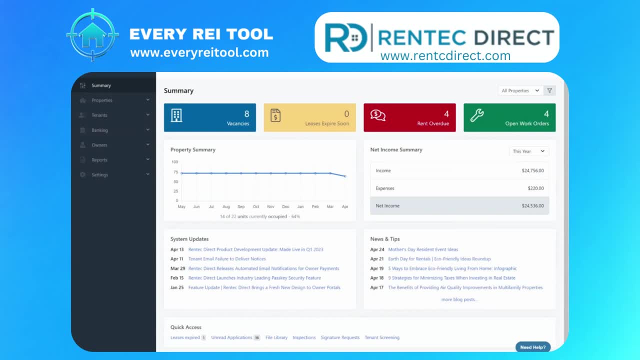 You can set up, uh, all, your, all, your chart of accounts, from your advertising to commissions, repairs, et cetera. You can create, add, subtract any of these that you want And, in our accounting platform, like many others, um, all your reporting is going to be based on these. 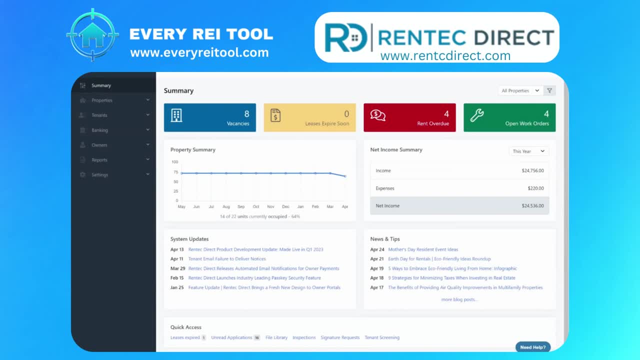 Particular accounts. you want to know. you know how many repairs? uh, so if we were to go over to our property here and we were going to post an expense to expect a single family here, we'll do this. one, two, four, test street. 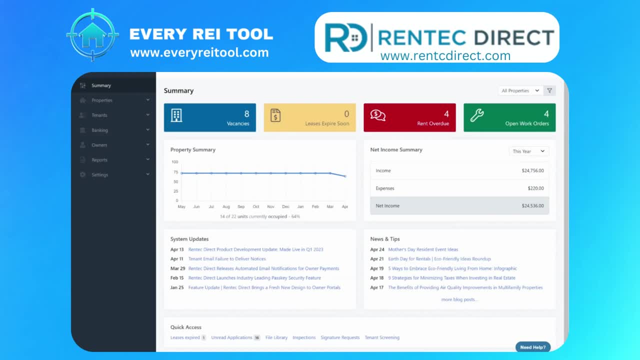 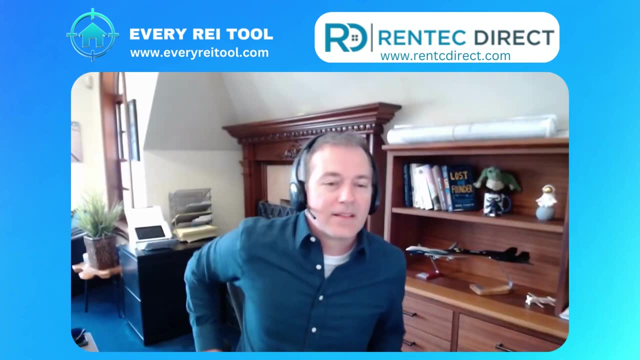 Go ahead. Yeah, Nathan, I think we're still seeing just the rent tech direct uh landing page, So I don't know if you went to a different tab. Oh sorry, Yeah, Let's see if I can bouncing all around and you're just looking at the same thing here. 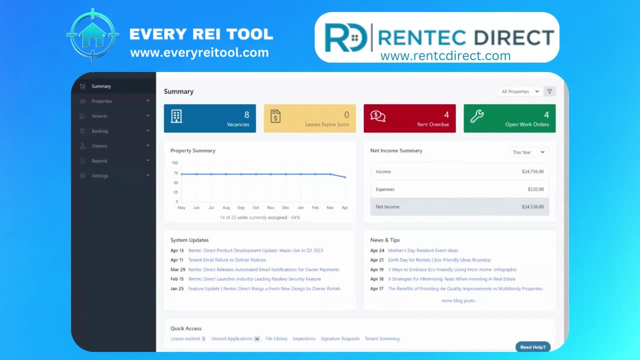 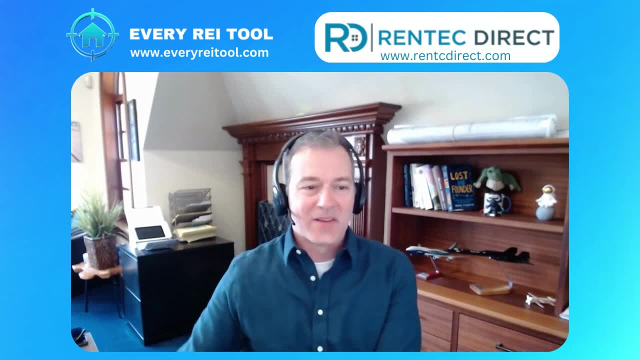 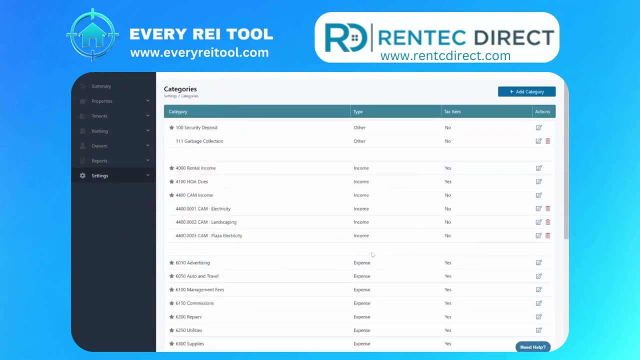 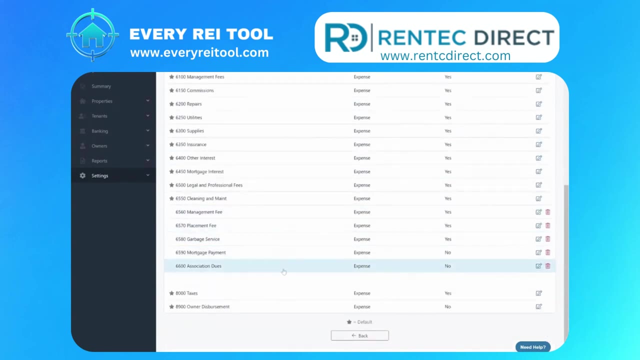 This tab instead. Perfect, Okay, Sorry about that, Let me. let me bounce back over there to that chart of accounts. So under settings, uh, all of our income expense categories- um, here's all the stuff you would look to see, everything that start or kind of your defaults, and then you can add, delete, subtract anything else you want in there. 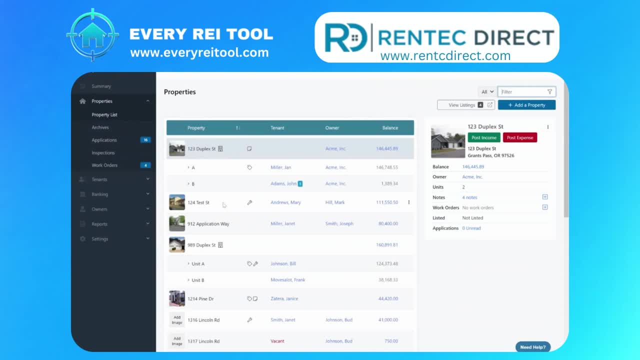 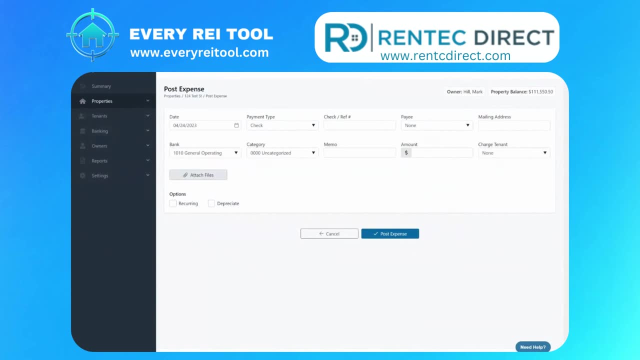 So if I were to go over to one of our properties here- this one, two, four test street- and I'm going to post And uh, let's just uh, put in some information here, let's make it a um, a repair. 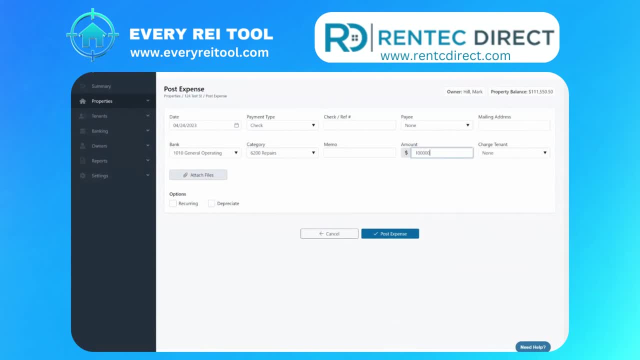 And so it stands out for this demo. I'm going to make it a $100,000 repair and a big repair. this it's a- yeah, we're going to call this a- uh, I dunno- a rebuild. How about that? 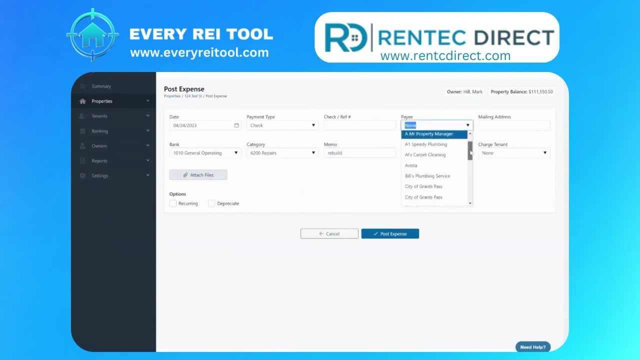 Yeah, And uh, let's, uh, let's see here Who's who's it going to? um well, it's a carpet, it's a lot of carpet, It's a carpet, Let's do it. 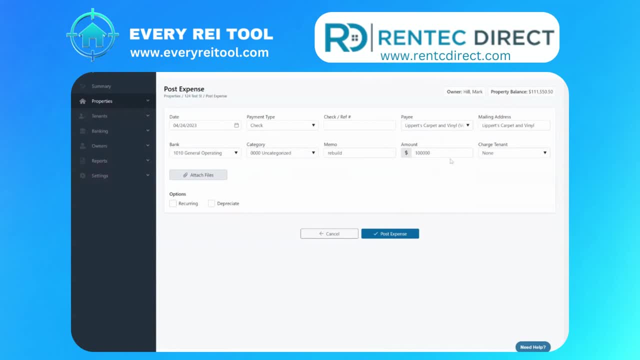 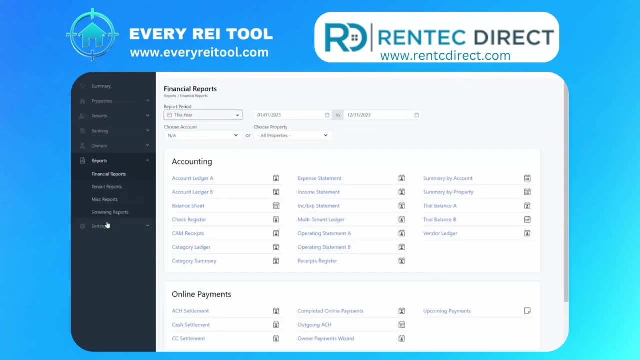 It's a carpet. Yeah, absolutely alright. so I'm gonna go just go ahead and post that expense and I'm gonna show you that was on 124 test Street. so if we were to go over to reports and we run an income expense report, I'm gonna select, I'm just gonna. 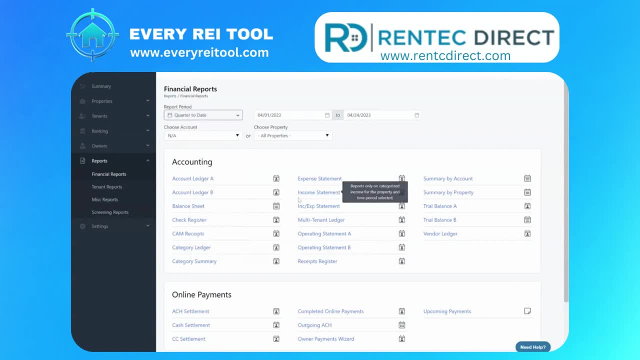 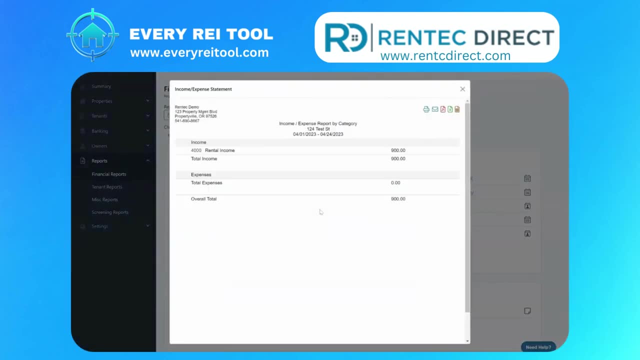 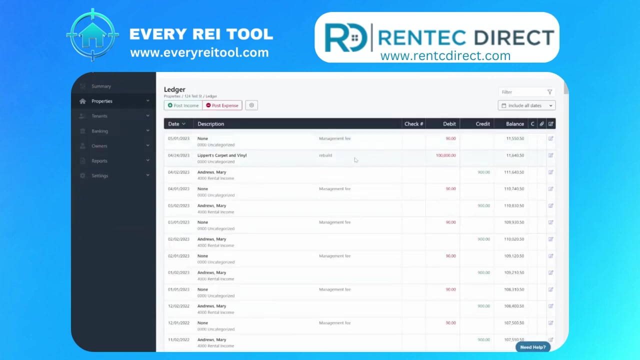 do this quarter, since we just put it for today, and let's do this one, two, four test Street, so it's not a huge report, and let's go find out where, where I actually put it. I might have picked a different date. okay, we did 424. oh, let's. 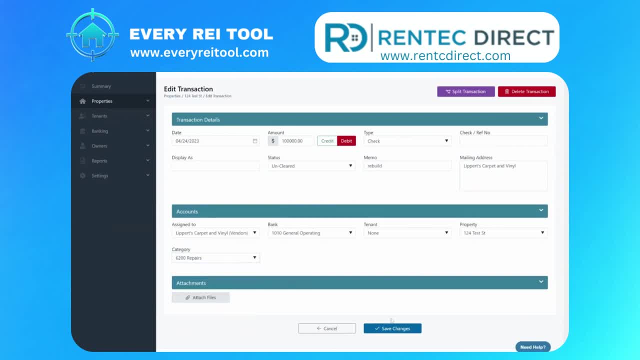 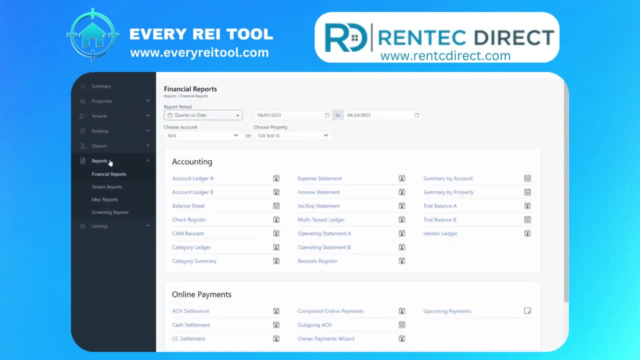 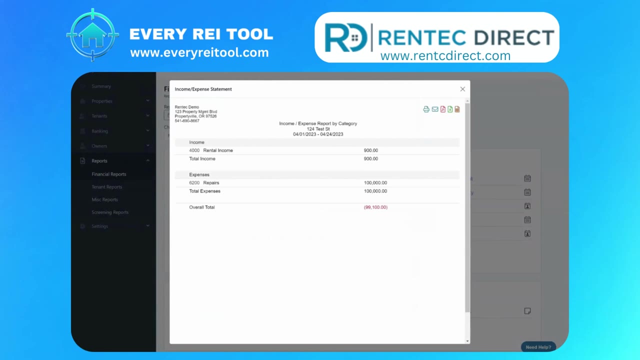 go. that's better. now it's showing up in repairs. that's all we needed, got it. yeah, okay, go back to our income expense. all right, now we have a giant $100,000 expense. yeah, your income expense reports. I mean, these are that and the Schedule E, assistant report. 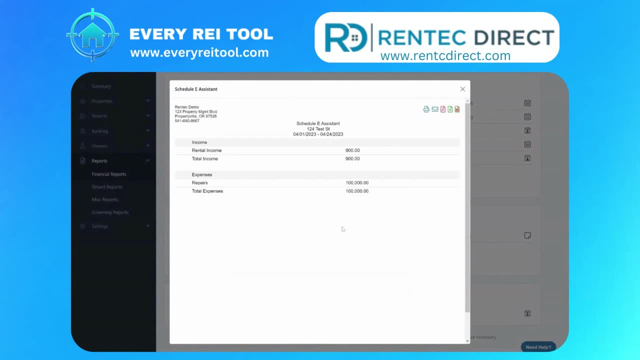 when it comes to tax time, this Schedule E report is probably the key to making your taxes simple. your CPA he wants, he wants one of these for each one of your properties. so I was literally just asked that last week. I was literally just asked that last week. 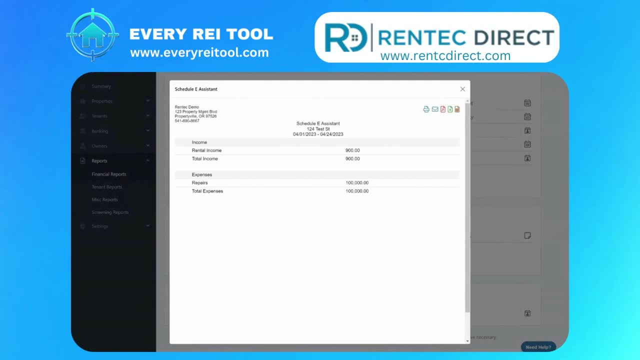 I was literally just asked that last week. you bet every bit of income and every bit of expense is categorized exactly the way they need it and you can even exclude categories from this report if for some reason you needed to. generally not wise, but the program gives you that. 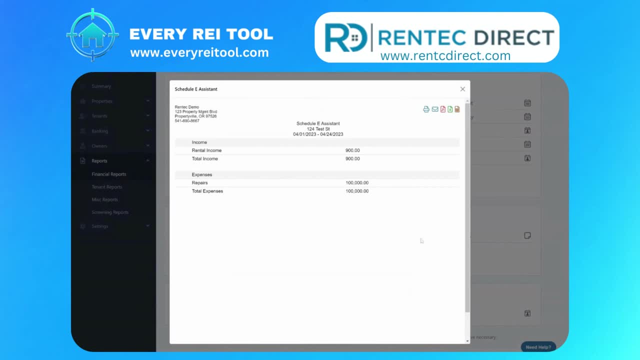 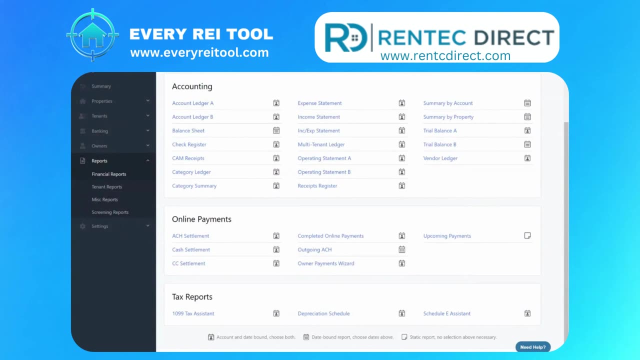 kind of flexibility to be able to do that very cool. yes, that's what makes taxes really easy. what else could I show you in here, Nathan? well, I mean that's already. I mean a great overview here, and I love how one thing that stands out, to me at least, is: 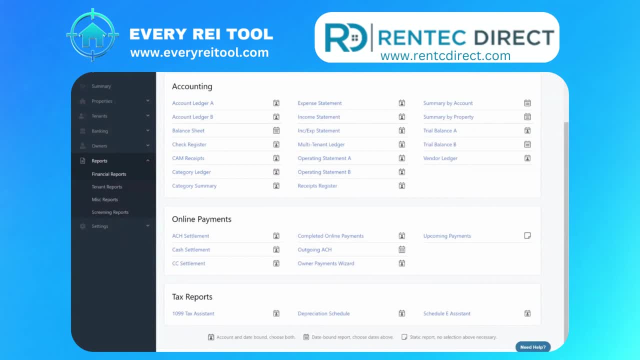 just how clean and simple it looks and seems to be to use right. I obviously can't claim I'm using this now, but I mean it's wonderful to see how easy it you know looks and seems to be right. So that's awesome. Great job on that one. I'm just curious. maybe last question here before. 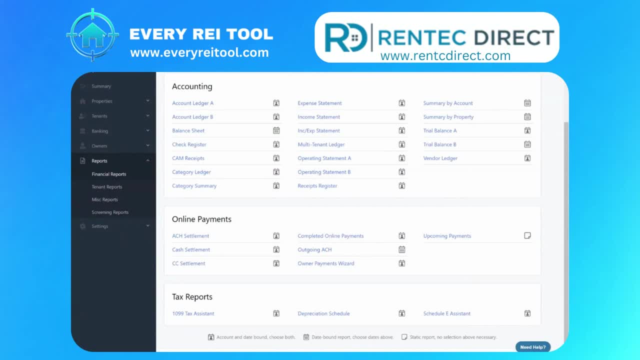 I let you go, Nathan, I want to be mindful of your time, but would you say your customer base? is it more owners or like property managers of like portfolios? Do you know what it is? I'm just curious. I do, And I'll tell you it's changed a bit over time because back in 2007, I made this. 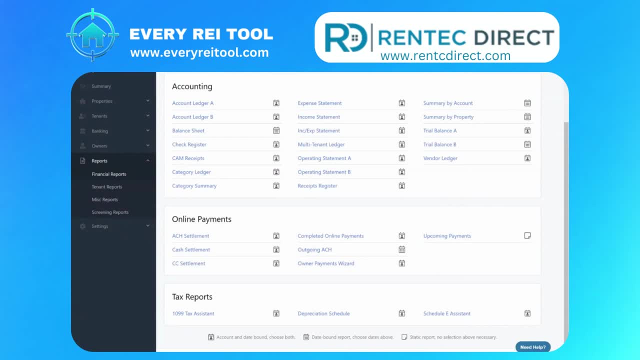 program, just for sorry for landlords, because that's what I was. I had a handful of properties made the program with me in mind, took some other landlords modeled after them too, to kind of create the features they need. And it was just a free program. I was just going to give the thing away and I did. And then we had